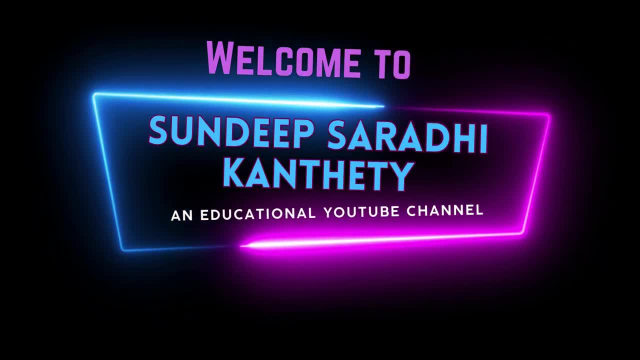 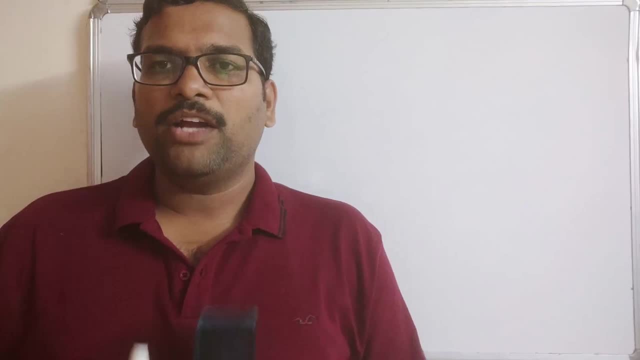 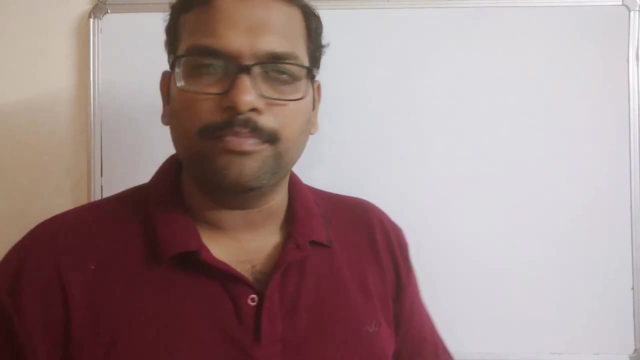 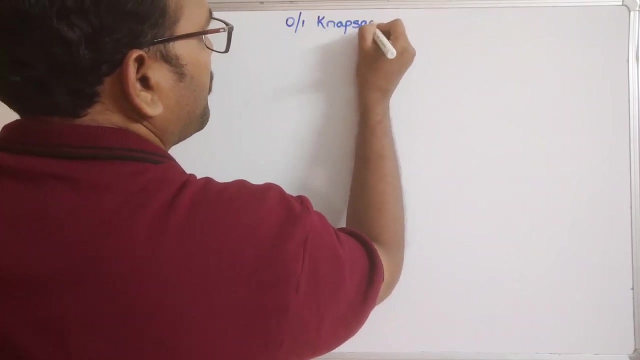 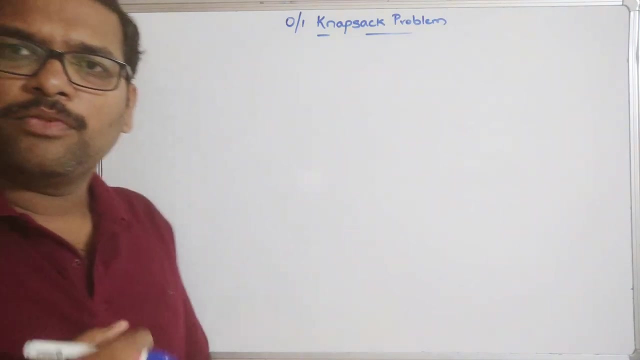 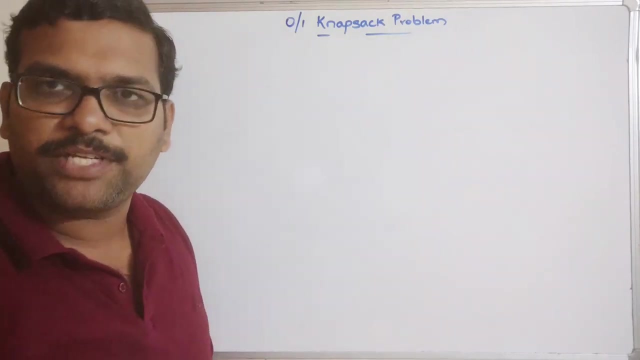 Hello friends, welcome back to our channel. So today we will see one more concept in algorithms, concept that is 0-1 knapsack problem. 0-1 knapsack problem. So before going to this problem, first let us understand what is meant by knapsack and what is meant by 0-1 knapsack. 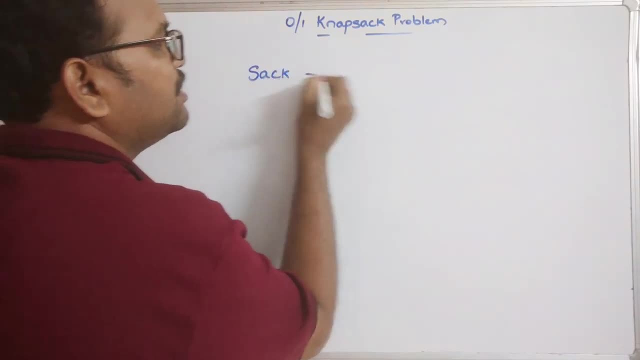 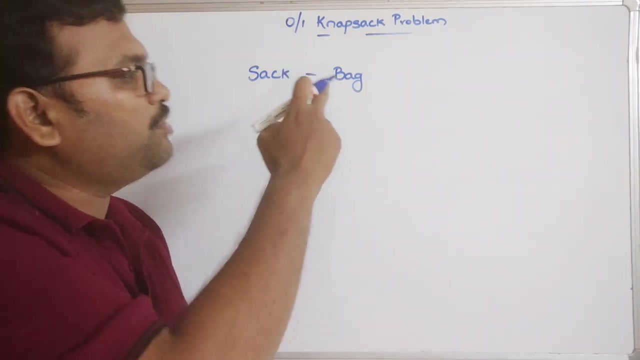 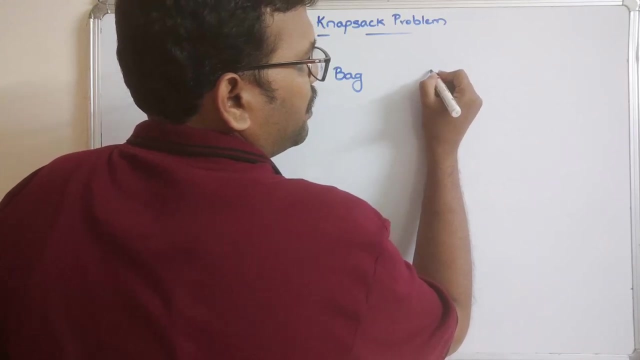 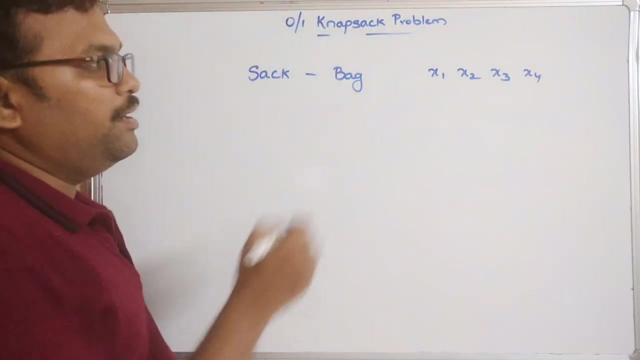 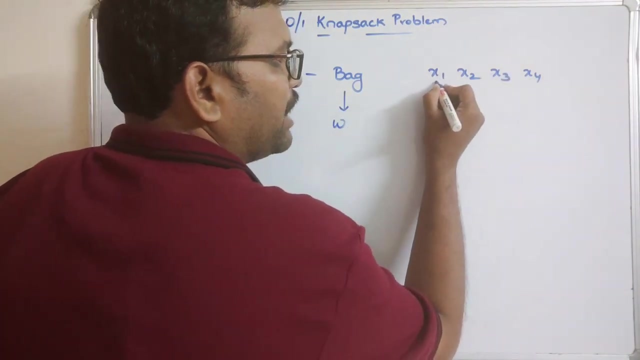 So we know that a sack- sack means it's nothing but a bag. So here the problem is: we are supposed to fill some objects into that bag with a highest profit. So let us consider four objects, right, Some x1, x2, x3 and x4, and the weight of the bag is w. Okay, so these are four objects and for each, 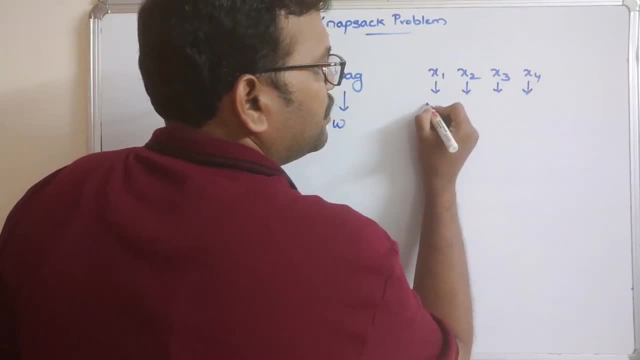 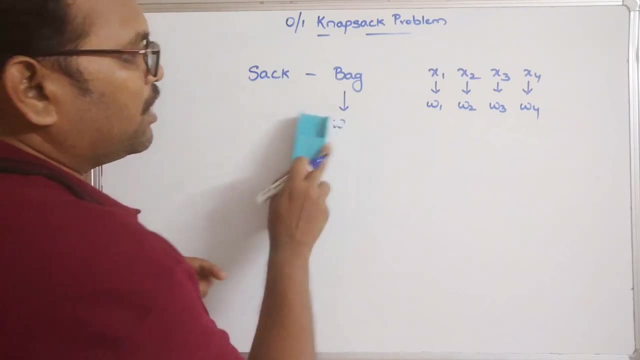 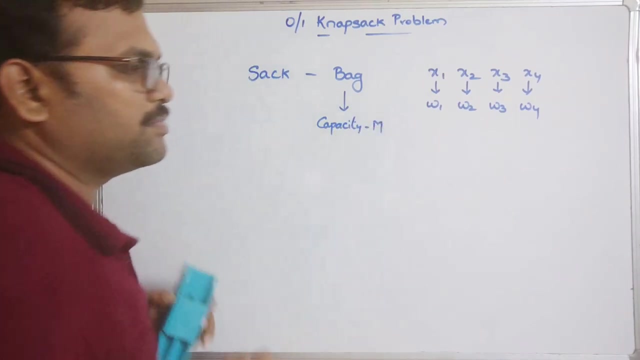 object. there will be different weights, So w1, w2, w3, w4.. Okay, in order to avoid the confusion, let us take the capacity of bag. Capacity is represented as yam, some yam. Okay, so there is. 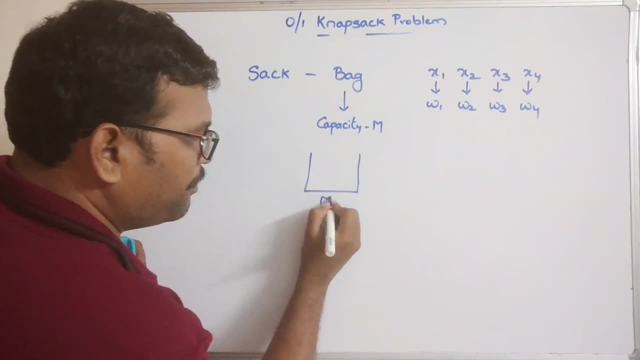 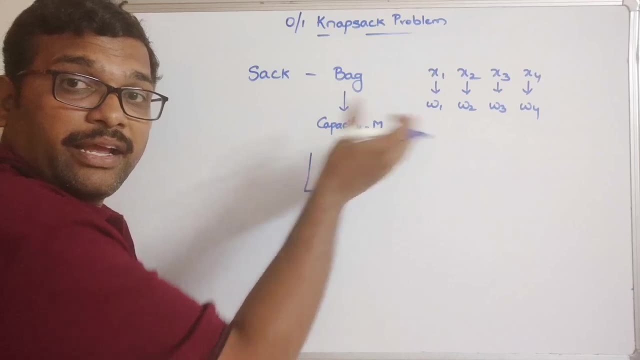 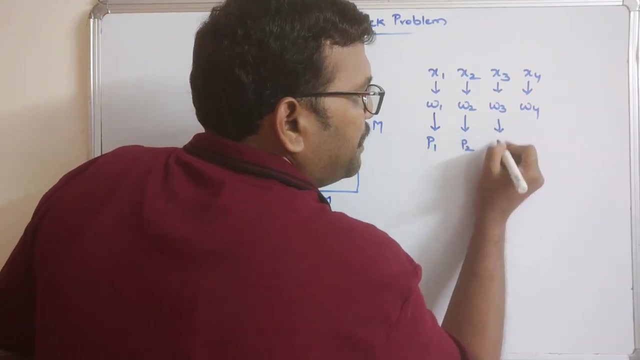 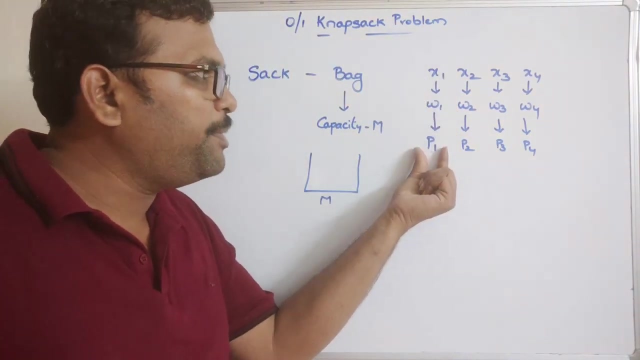 one bag or one container with a capacity- yam- and here, in order to move these weights into the bag and carry towards somewhere, it requires some profits. So p1, p2, p3, p4.. So with this particular x1, we will get a profit p1.. With object x2, we will get a profit p2, x3, p3 and x4, p4. 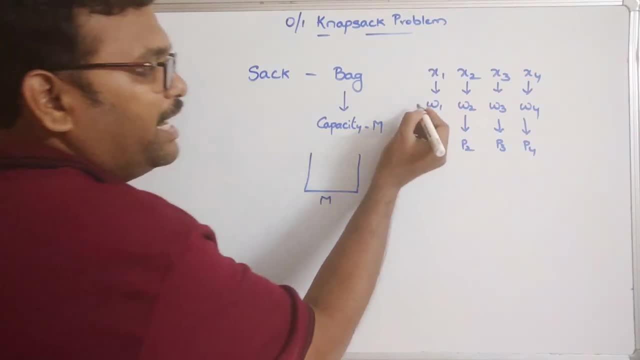 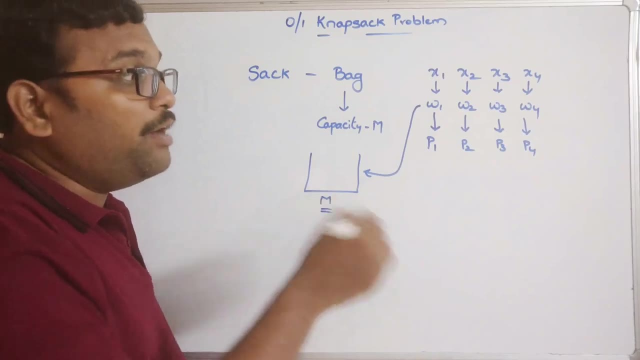 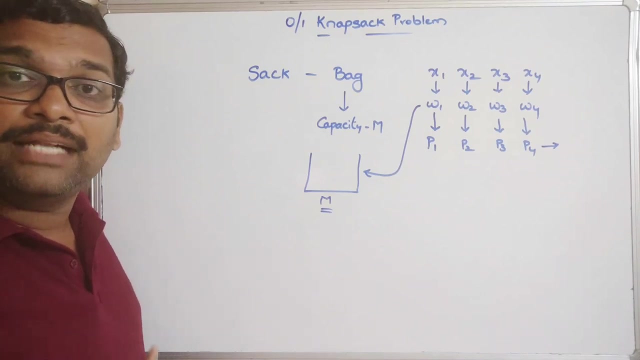 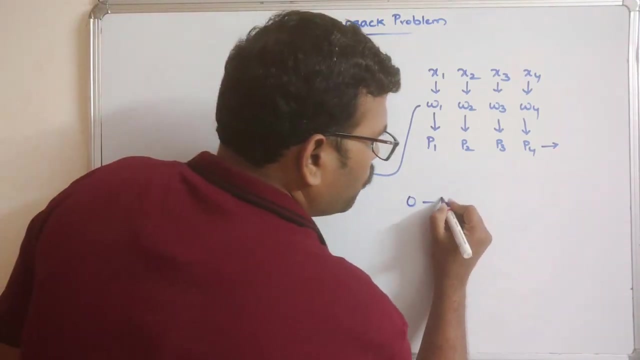 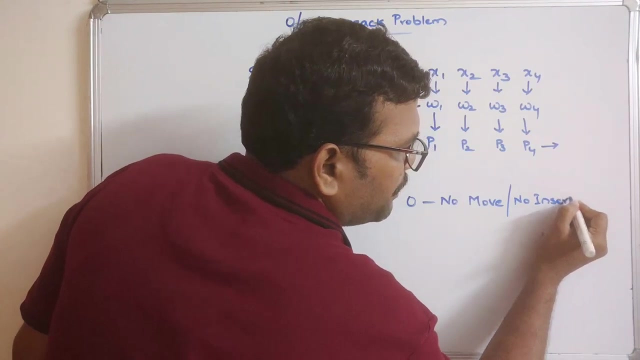 Here. the problem is we have to arrange the weights into this particular bag. that should not exceed the maximum size And we need to get the maximum profit. That is the problem And why we are calling it as 0 and 1 means here. 0 indicates no move or no insertion. That means we are not supposed to move the weight. 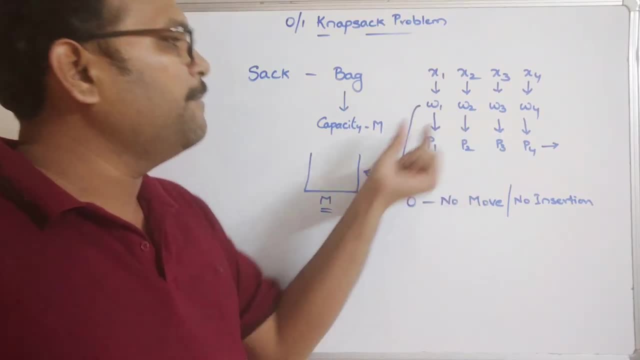 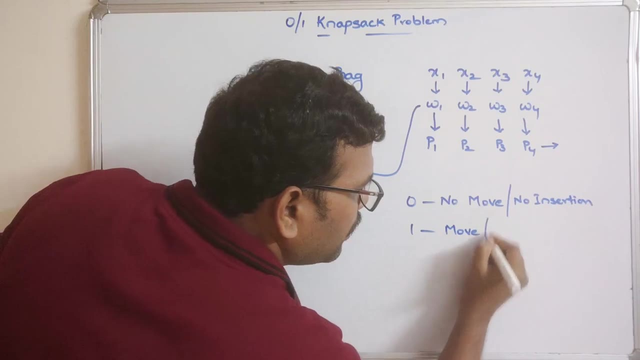 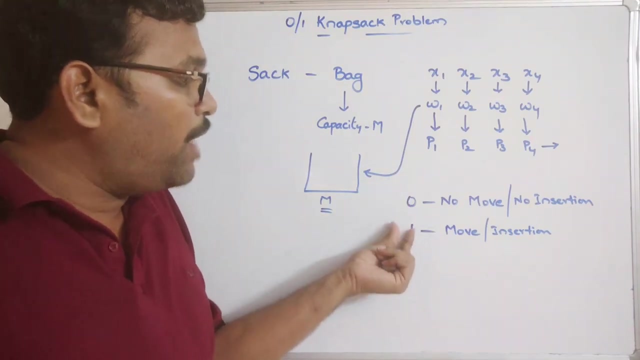 into this particular bag or we are not inserting the particular bag, We are not inserting the weight into this bag, And 1 implies move or insertion, Move or insertion. So that means if 1, 1 represents moving the weight into the bag. 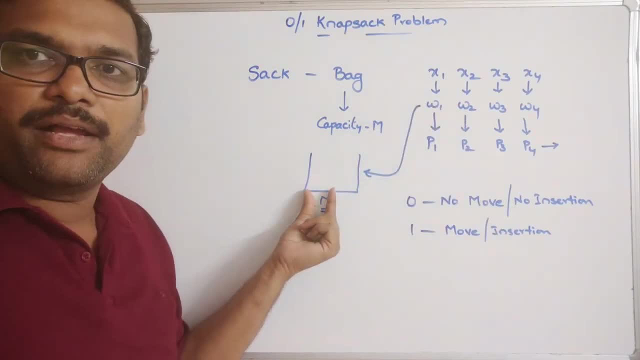 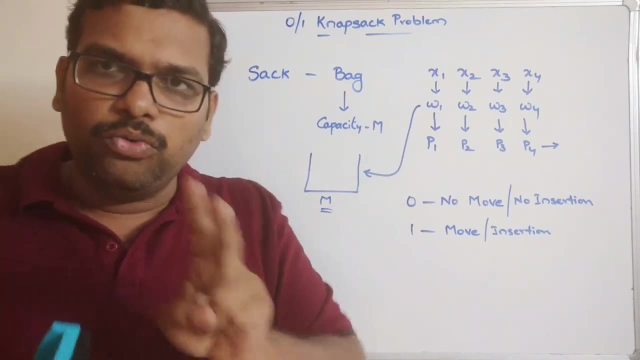 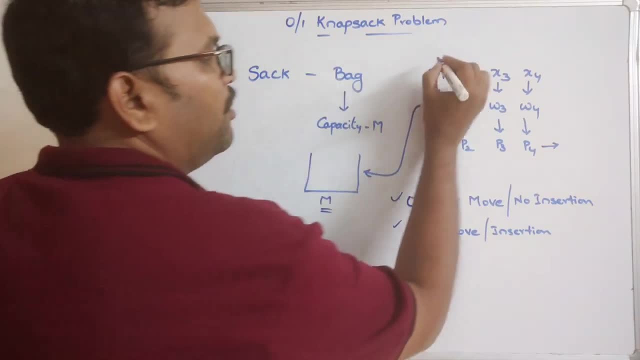 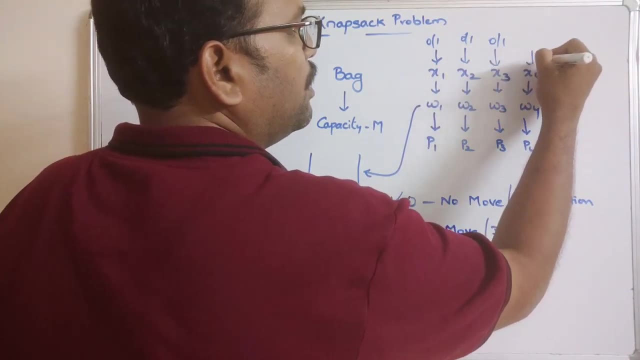 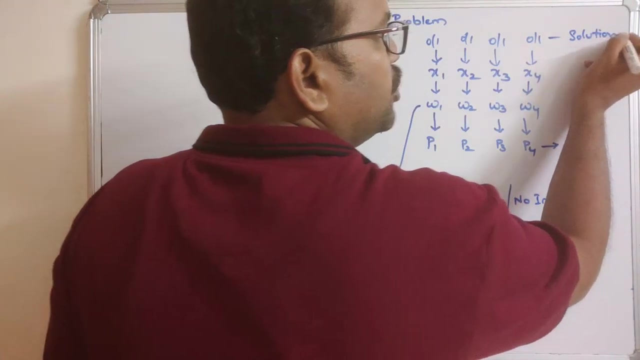 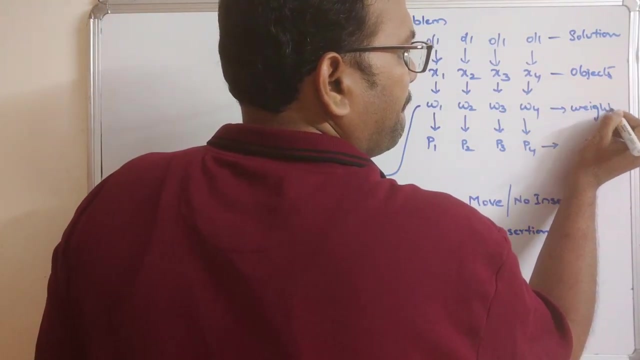 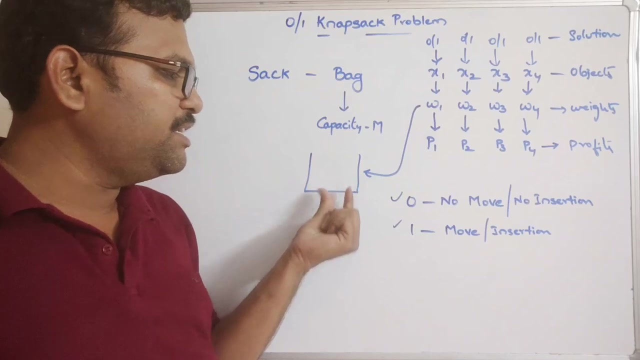 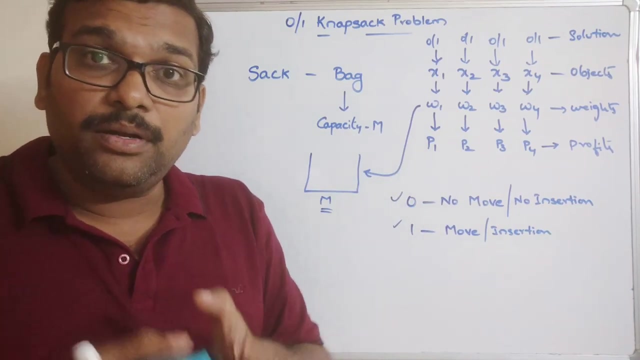 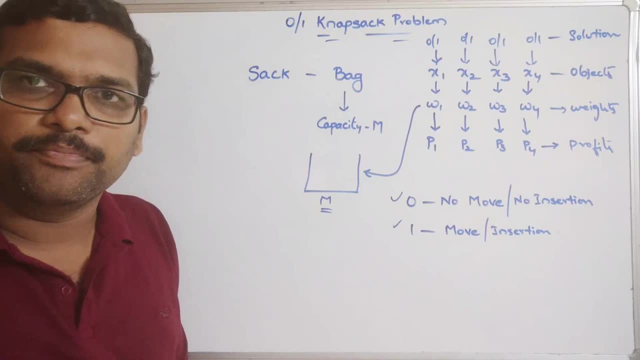 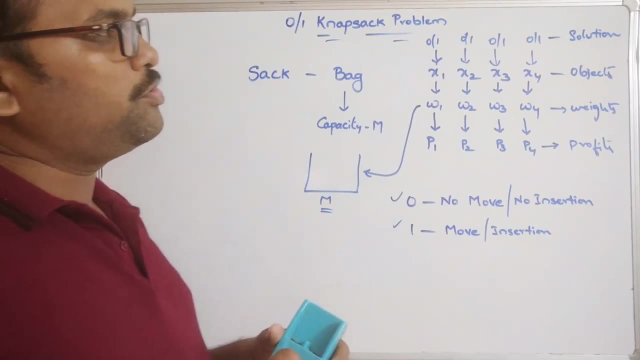 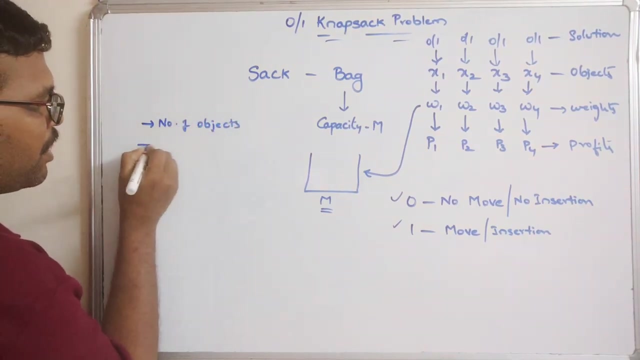 So that's why we call it as a knapsack problem, Knapsack problem. So in order to solve this knapsack problem, we are supposed to have the four things: One is number of objects. Second one profits: weights, capacity of sack or bag. 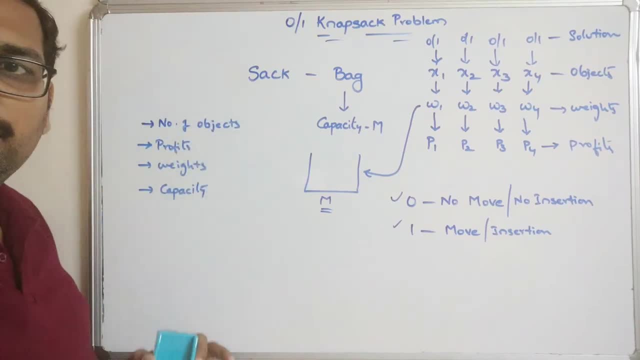 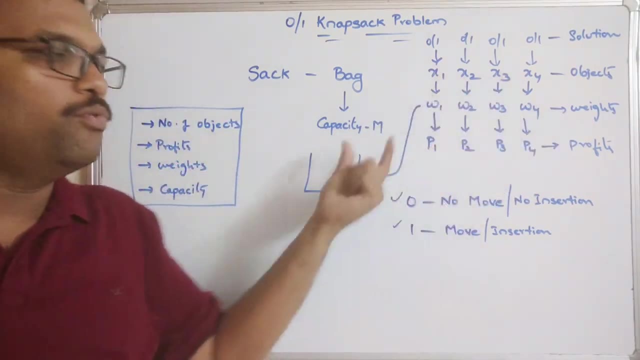 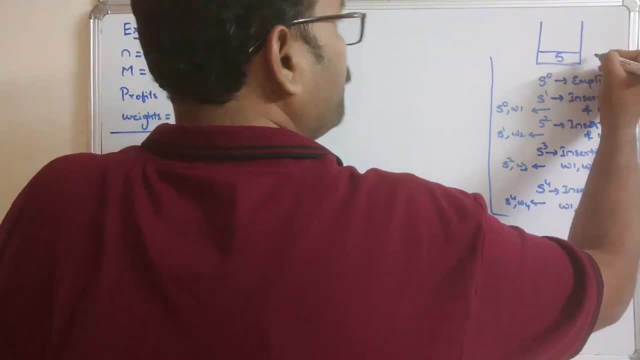 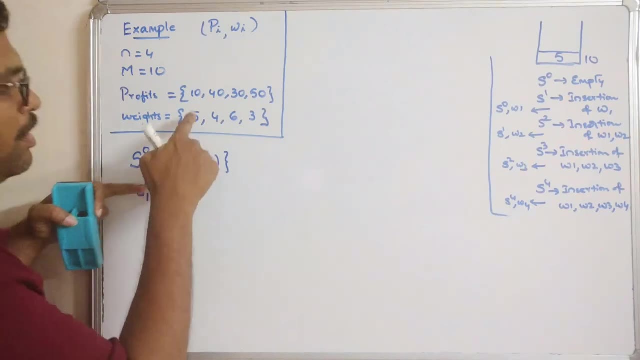 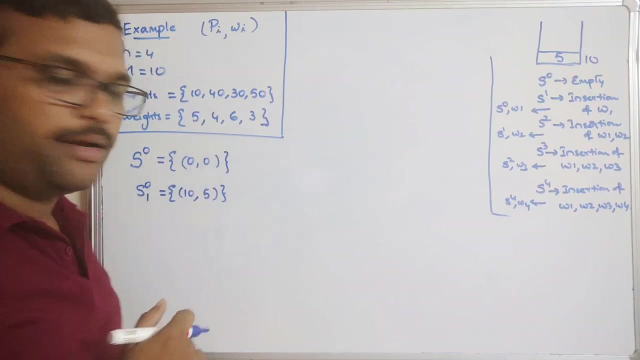 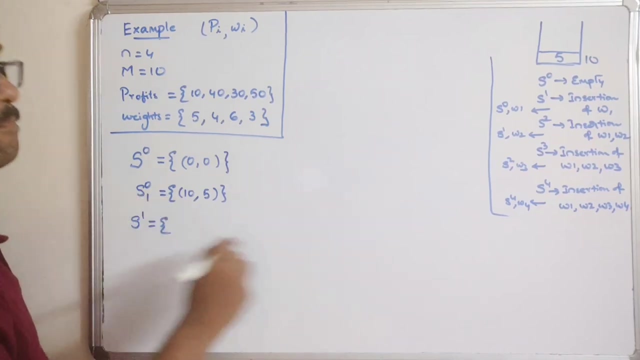 So if you are having these four things, we can easily find out which objects should be moved from outside to the outside the sag with a profit 10, so 0 plus 10 comma, 0 plus 5. okay, we have inserted now what is the s1- yes, one, yes, one will be. what is s1- yes, not. and w1, so yes, one. 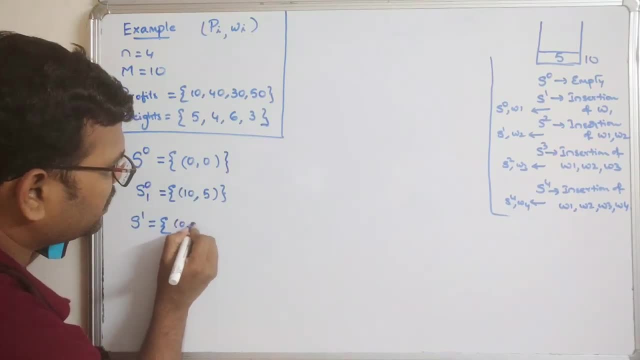 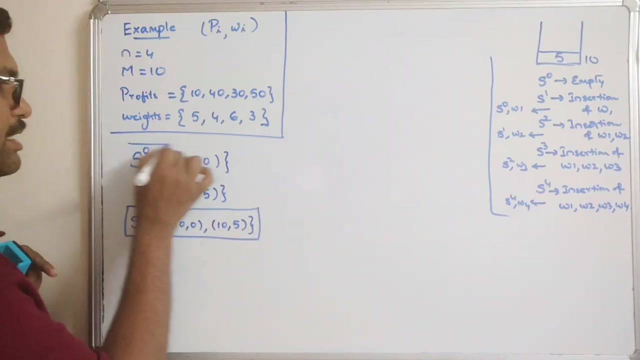 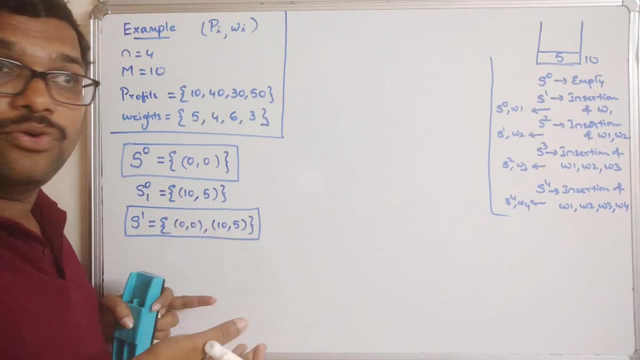 means s, not means 0 comma, 0. yes, w1 means after insertion of one thing. so we are getting 10 and 5. so this is the yes one, remember this one, you. and this is yes, not okay. after that, what we have to do, we have to insert one more. 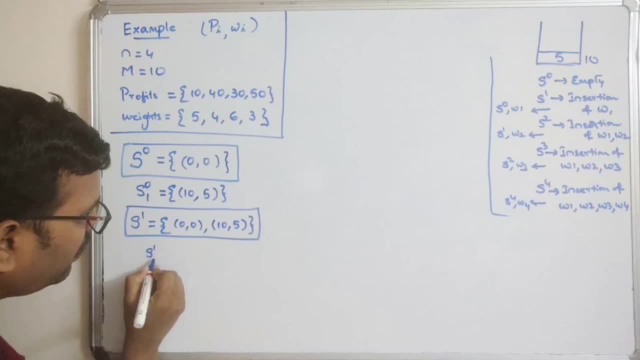 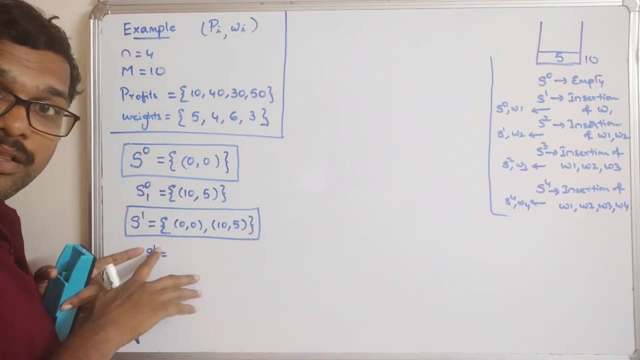 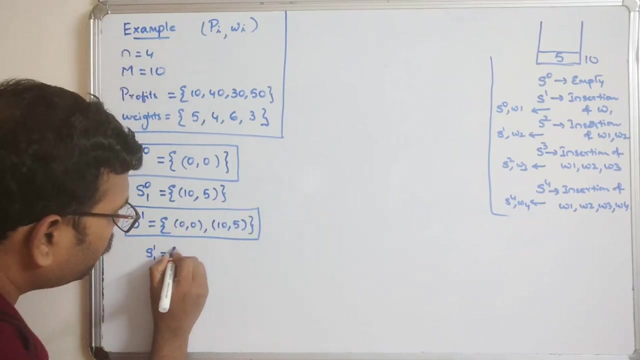 element right now, yes, one, and insert one element. so just remember the prefix. okay, the upper script will be the one and lower script will be the insertion of one element. so what we have to do, we have to add one more element. so one more element, and this is yes, 0. commappers say yes, kill other one, no cheat. 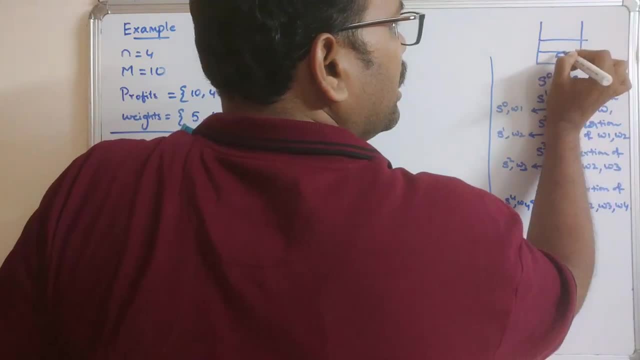 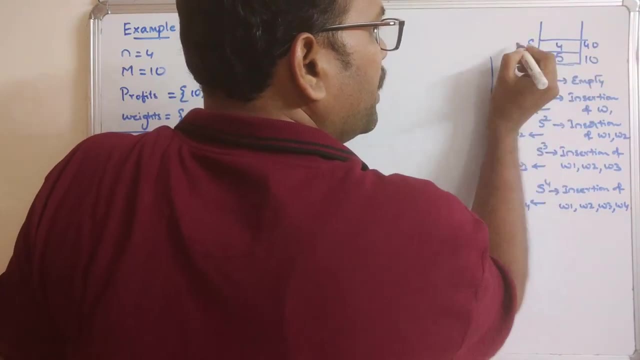 you have to do this, that's fine. so after insertion of one element, you have to: element means 4 with a 40. What happens here? If you add 4, okay, if you add a 4 and it is 40, what happens? So, complete it is 9 and complete it is 50, okay, The same thing apply. 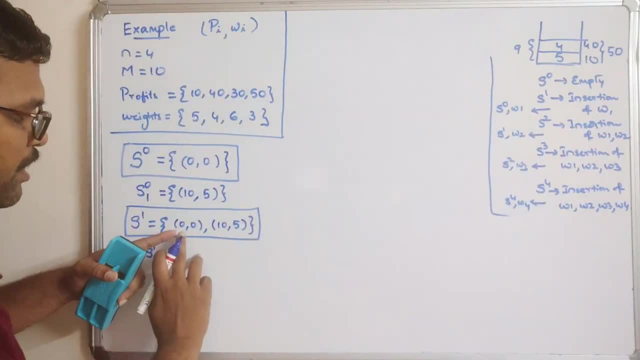 to the S1.. So S1, insert to S1.. So what happens? 40 and 4.. 40 comma 4, because we are adding to this particular S1.. 0 plus 40 and 0 plus 4 comma, Then combination: 40 plus 10, 50. 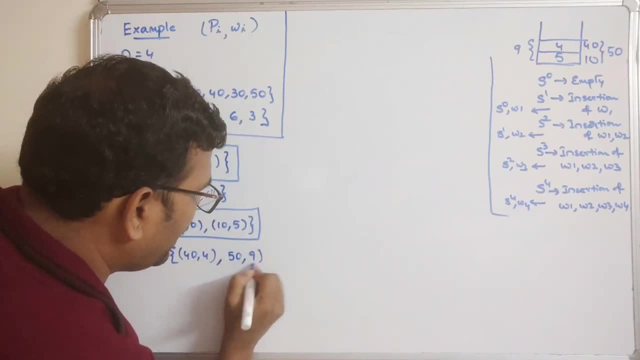 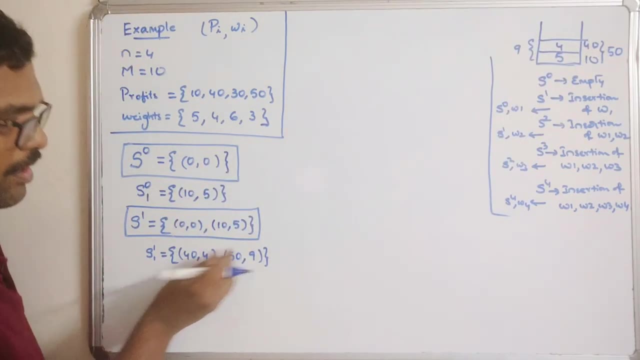 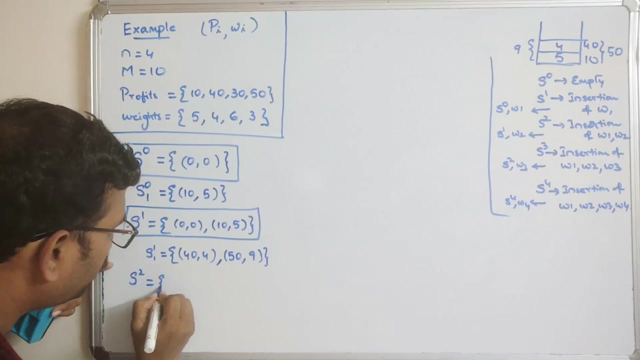 comma 4 plus 5, 9.. So you got it So empty Initially. we have moved it and then we are getting the next one. Now, what is a S2?? S2 is equal to. So what is a S2 here? S2 is equal. 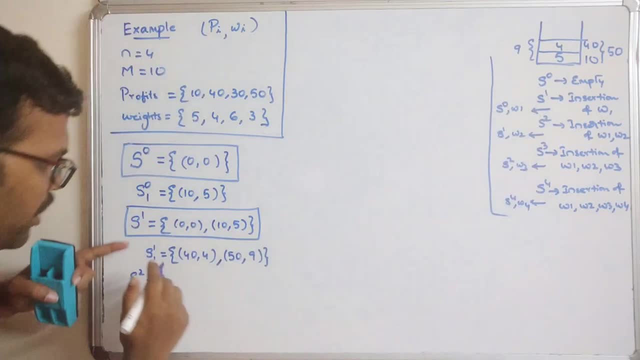 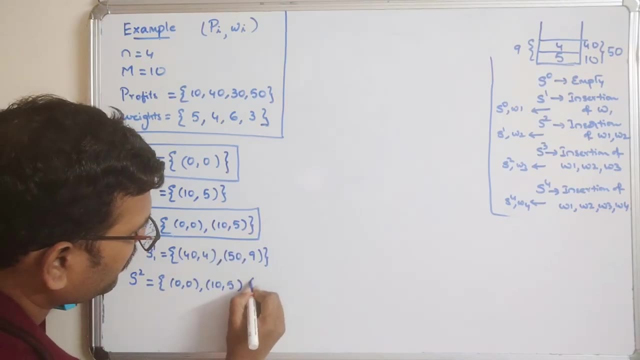 to S1.. So what is a S2 here? S2 is equal to S1.. So what is a S2 here? S2 is equal to S1.. So complete S1 and new thing. So S1 is here 0 comma 0.. 10 comma, 5.. 40 comma, 4.. 50 comma. 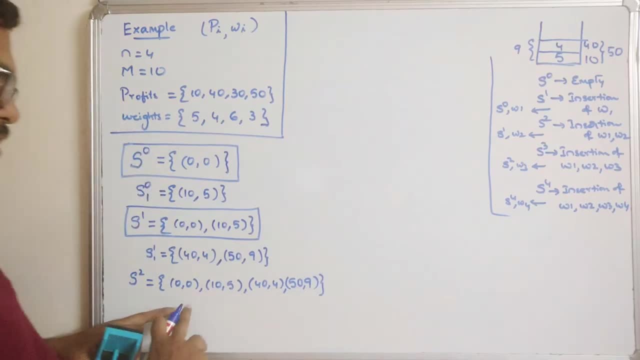 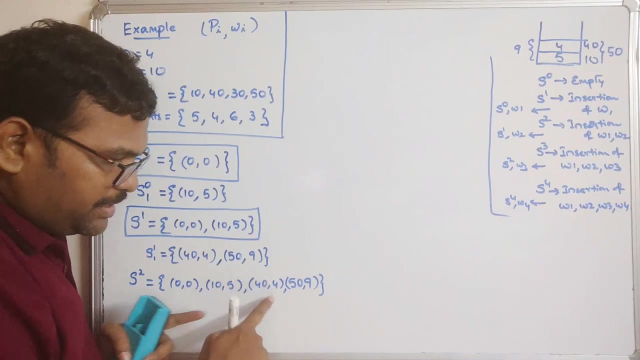 9. Right, Yes, Okay, Now you observe what it means: 0 weight, 0 profit. Okay, 0 weight profit with the zero weight. and if the weight 5- here we are having weight 5, how much profit we are getting? 10? good, second case: adding weight 4 and profit. 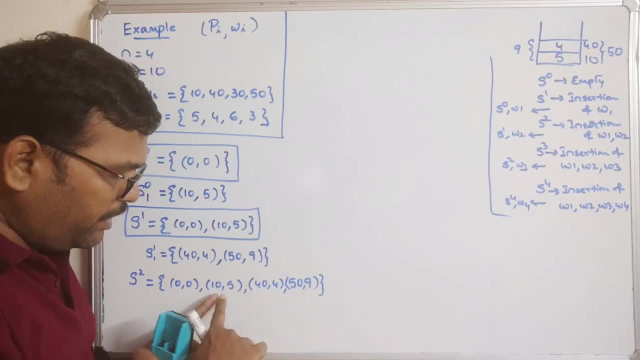 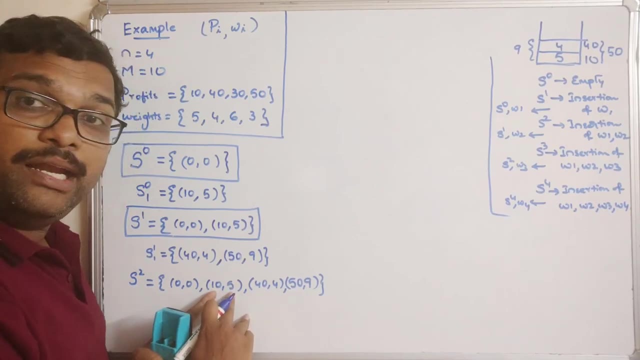 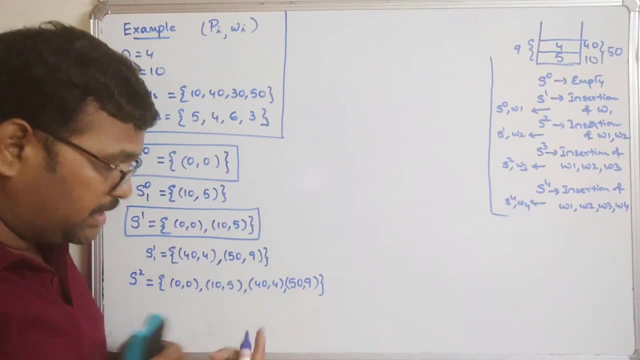 is 40. so you are getting less profit with 1 weight because you can see, with the weight 5 we are getting only 10 profit. with weight 4 we are getting more profit. so imagine it as a cages: for 5 cages the profit is 10 for 4 cages. 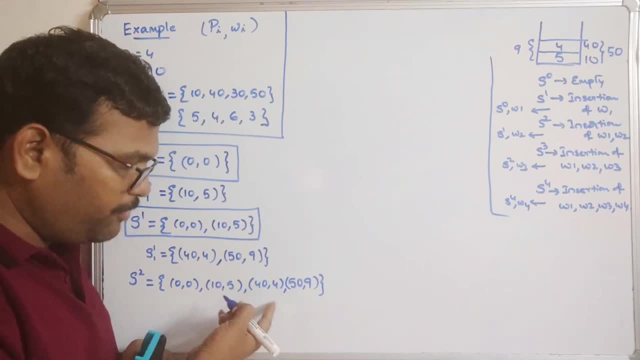 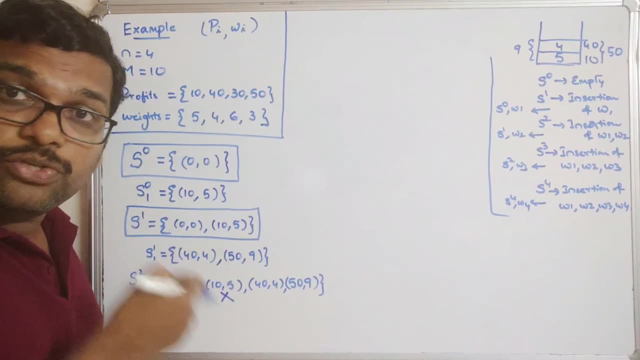 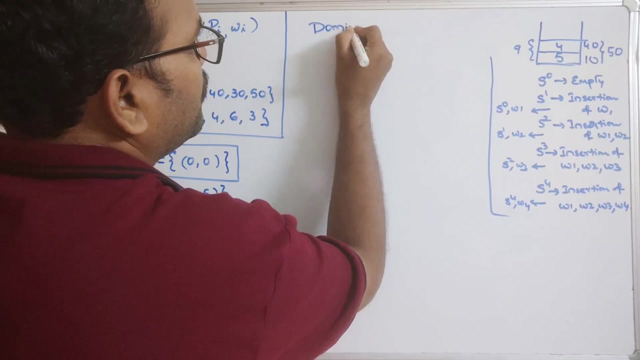 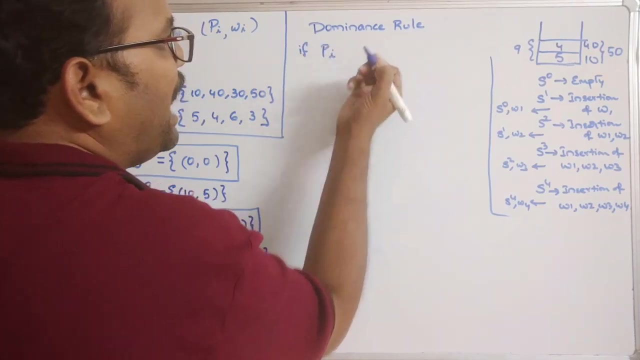 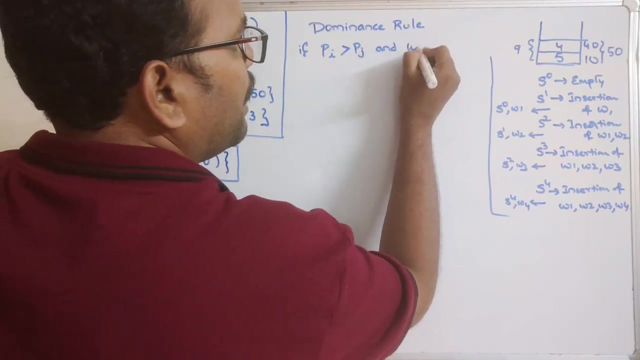 itself with the profit is 40. so which one is better? obviously this one is better, so we can avoid this particular case. okay, this rule, we call it as a dominance rule. okay, dominance rule. dominance rule, that means if PI is greater than PJ and WI is less than WJ, less than or equal to, okay, or? 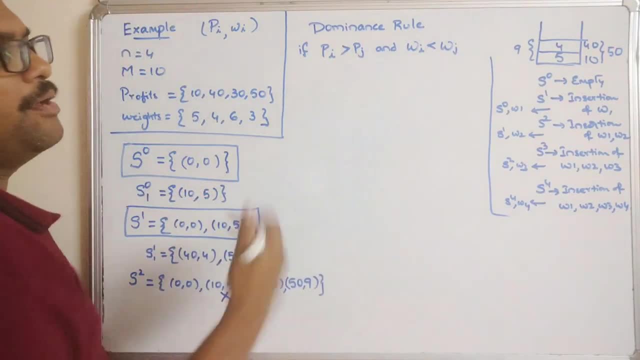 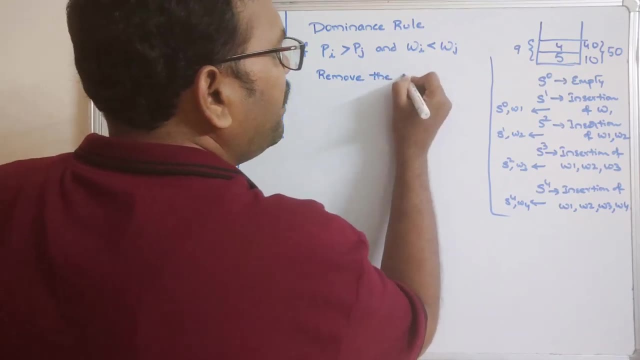 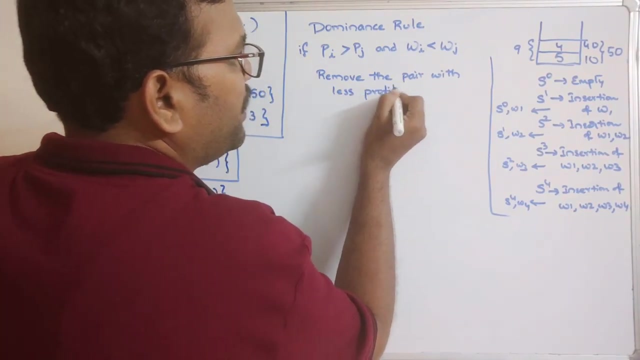 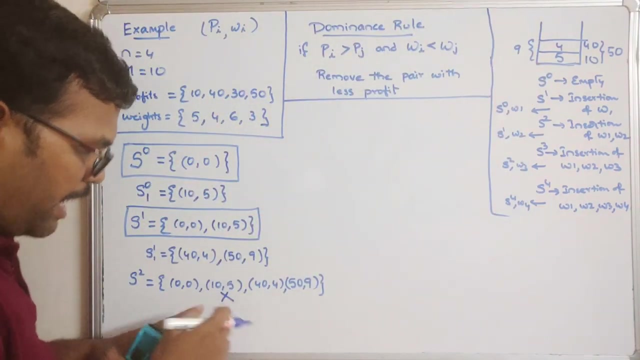 simply you can write it as less than okay, then we need to remove. we need to remove the pay with less profit, less profit. so this process we call it as a dominance rule. dominance rule: here the same thing happens. consider PI and WI, PJ and WJ: see PI, WI, PJ, WJ. what 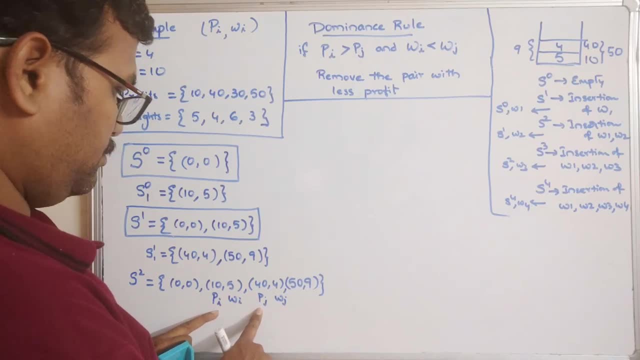 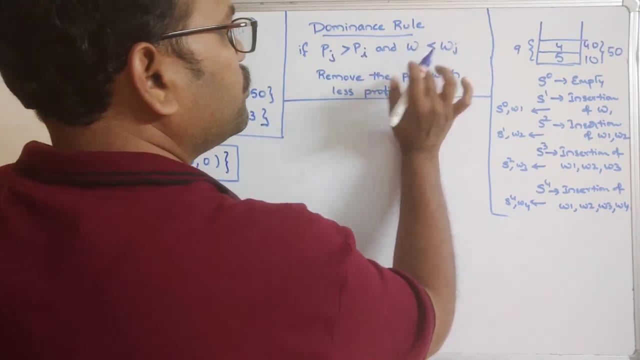 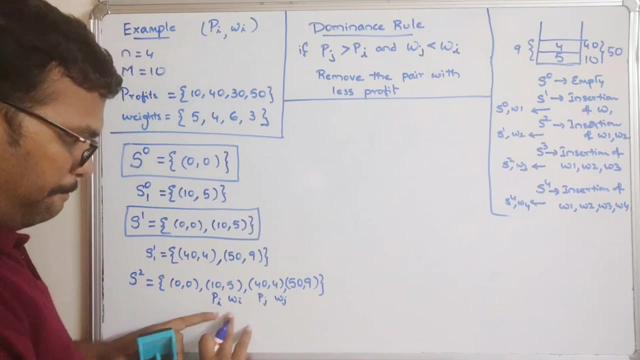 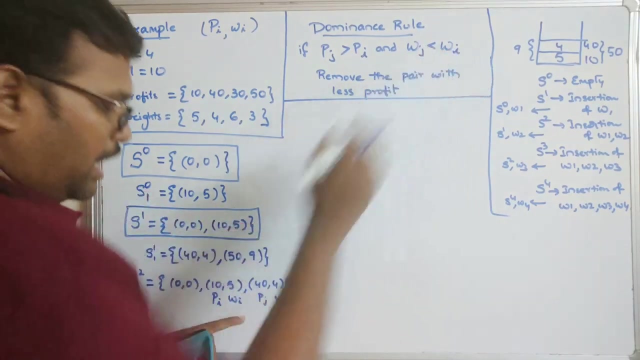 happens. PI is greater than- sorry, I have written small right- so PI is greater than PJ and WJ, PJ and I- and here also I write so increasing of weight should increase the profit. so PI, PJ is greater than P. I. PJ is rated an PA- perfect, and wj is less than WI. wj is less than W- I, so we need to. 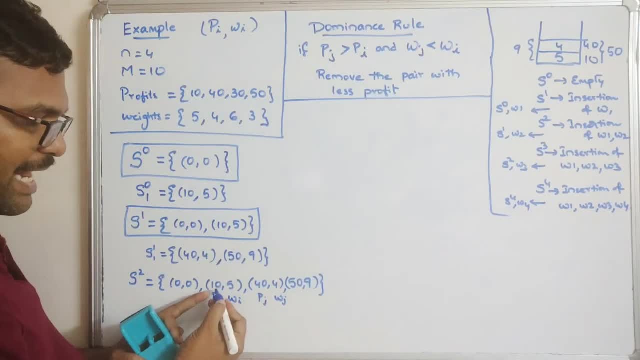 remove the pay with the less profit, which is having the less profit? n is the less profit, because the pain is profit to debate, not weight and profit. Don't get confused. profit is less than w? i and wait. The first term will be the profit, the second term is the wait. So if we need 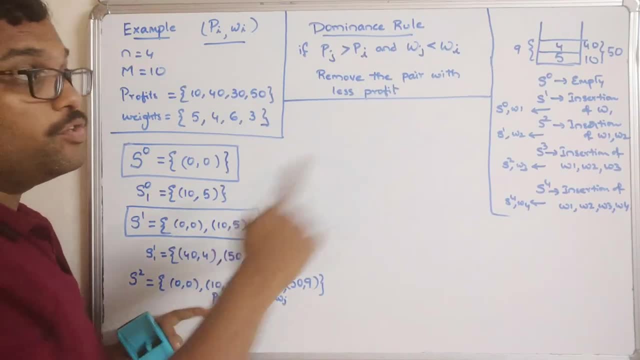 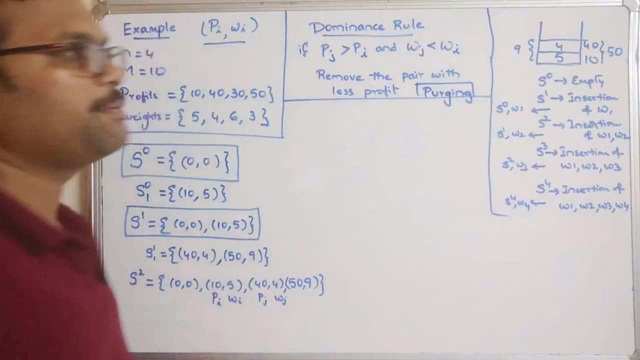 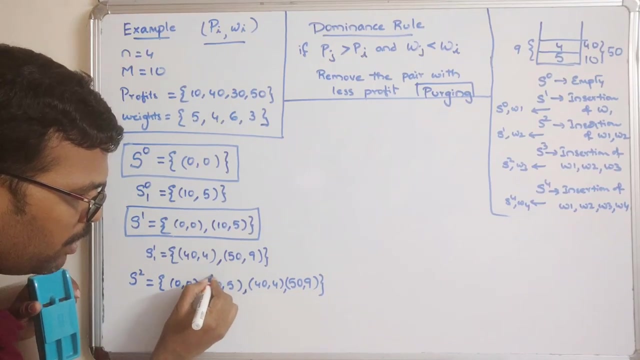 to remove the pay with the less profit, that is, a 10. So this is also called as a purging rule, Purging. Purging means removing, Also known as a purging Okay. So what we have to do in this case? We have to avoid this one. Avoid this one, Okay. So now we can. 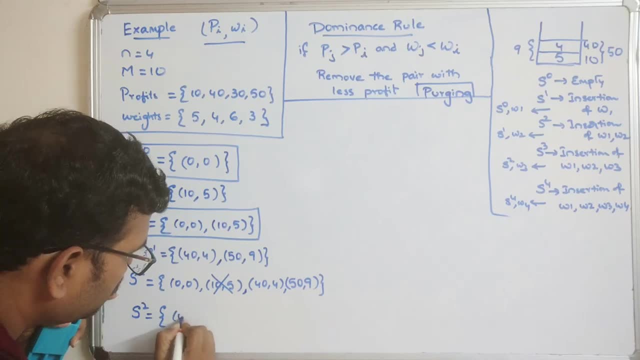 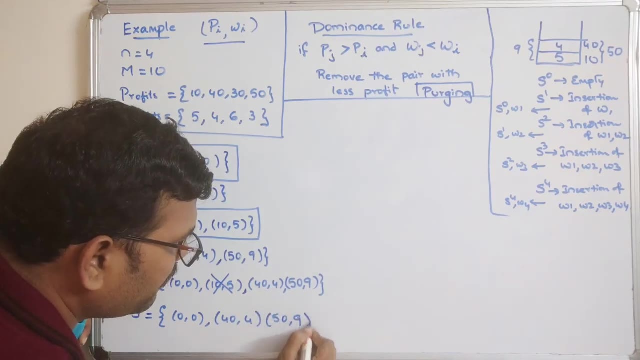 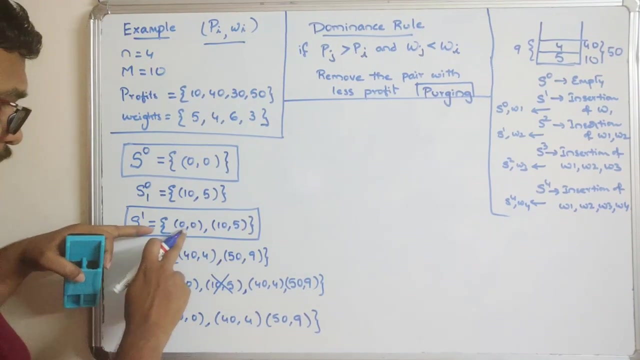 write the final S2, 0, 0,, 40,, 4, 50, 9.. Okay, Only 3 terms we are getting. So 0, 0,, 10,, 5, 44, 59.. So 10, 5 we are removing. So only 3 terms are there for S2.. 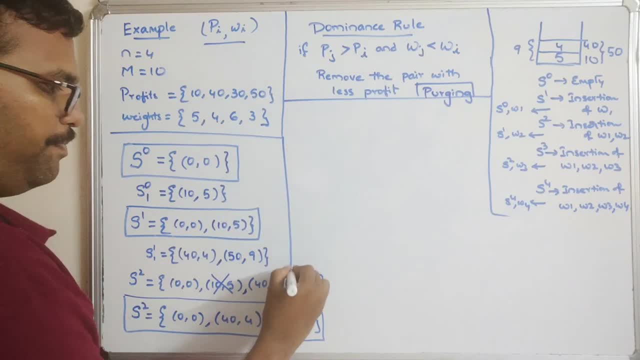 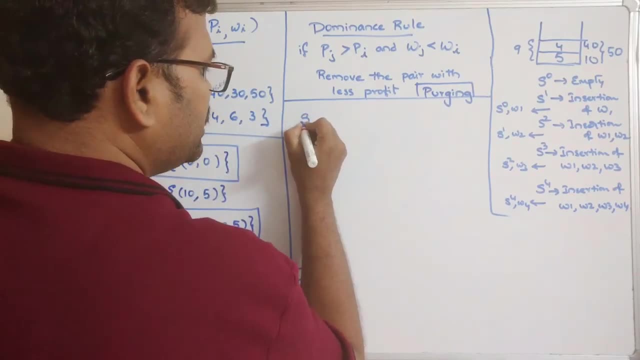 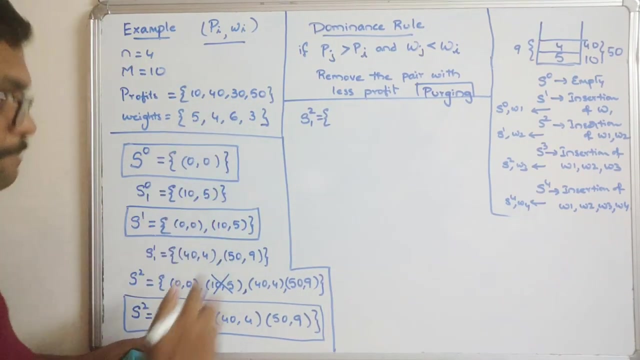 Now find out the next term. that is S3.. So in order to find out S3, we need to add 1 to S2.. 1 to S2.. So the next term is 30, 60.. So 30, 60. Sorry, 30, 6.. And add 30, 6 here. 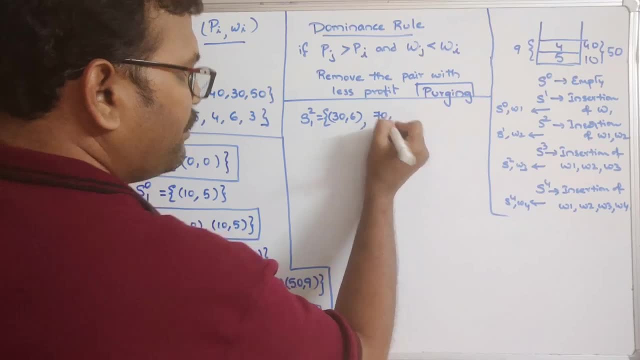 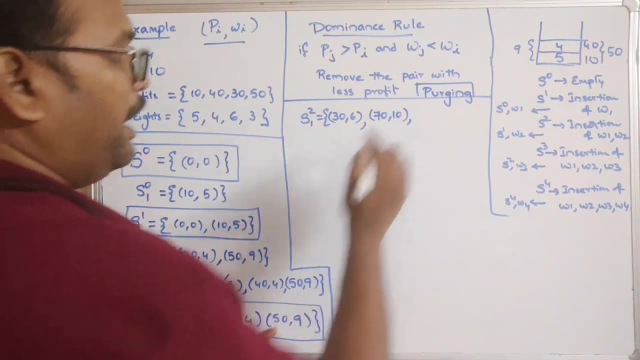 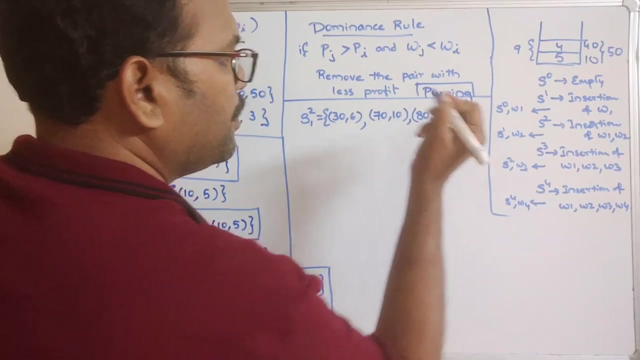 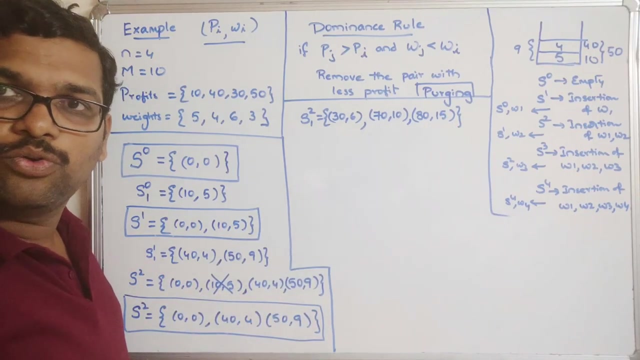 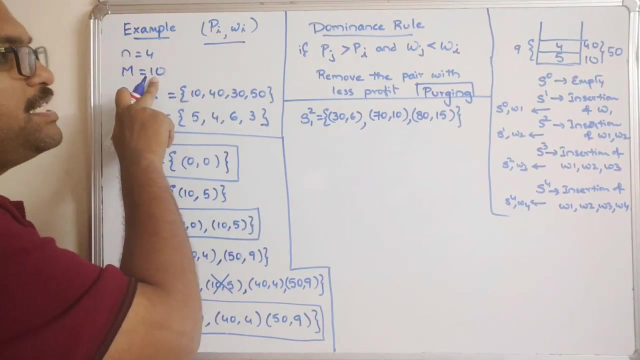 How much? 70,, 60., 10. And here 80,, 50. Okay, Now you observe, the profit is 80 if the weight is 50. That's good, But the maximum weight here is only 10. So in the 10 capacity bag we can't insert. 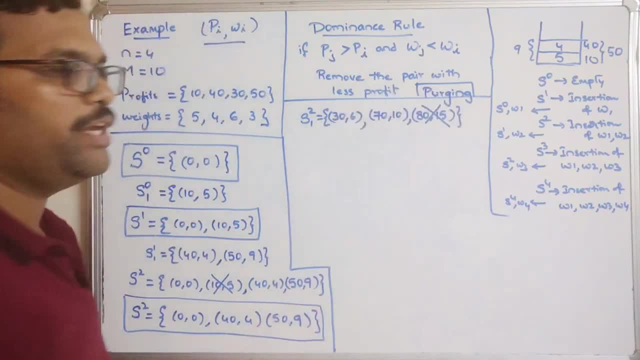 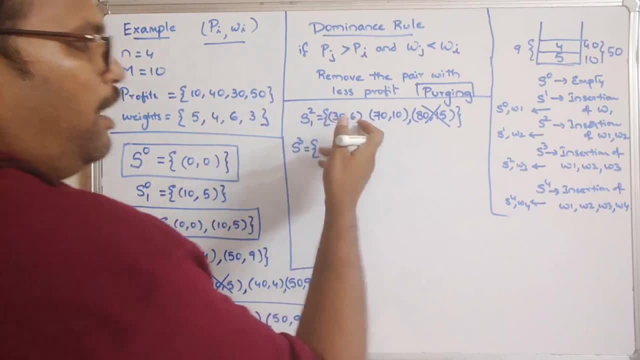 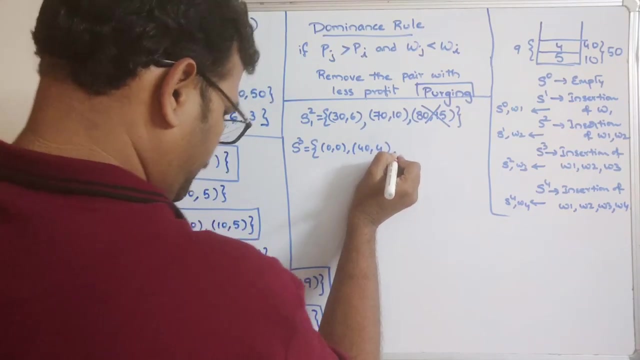 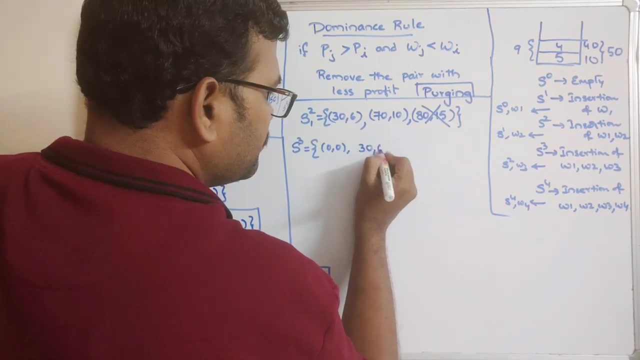 the 15 weight. So this is also invalid. So we need to remove that one. Now. S3 will be the combination of S2 and the insertion. So consider 0,, 0,, 40,, 4.. So before 44, we can get 30,, 6,, 40,. 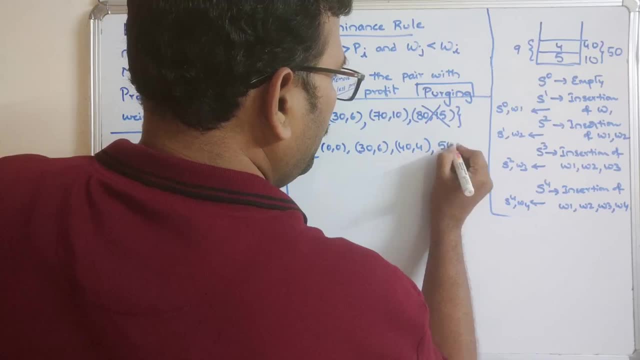 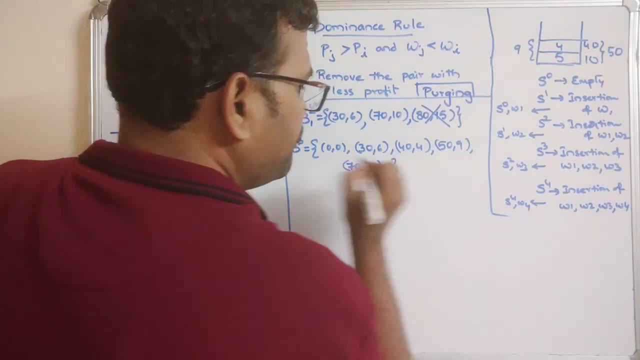 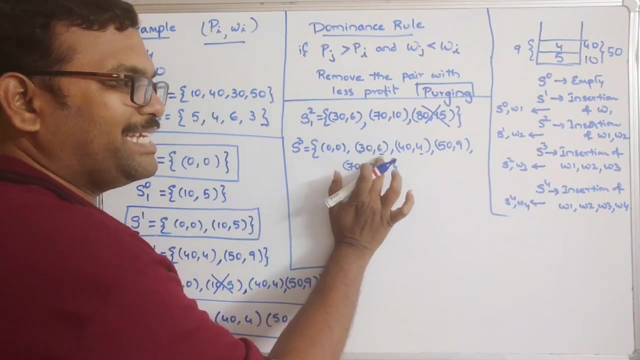 4,, 50,, 9. And 70,, 10.. So these are the elements. And now again you can see the same thing. So here 6 and here 4.. So we are getting a profit for 6, weight 30. And we are getting more. 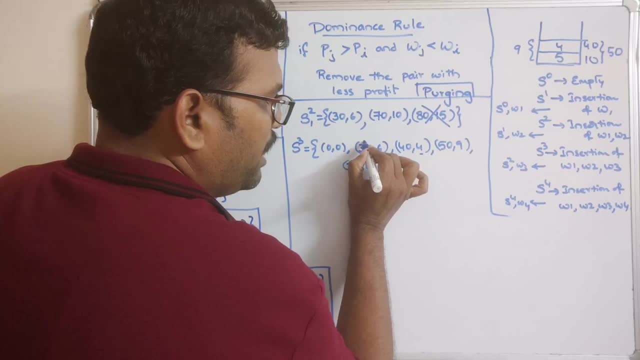 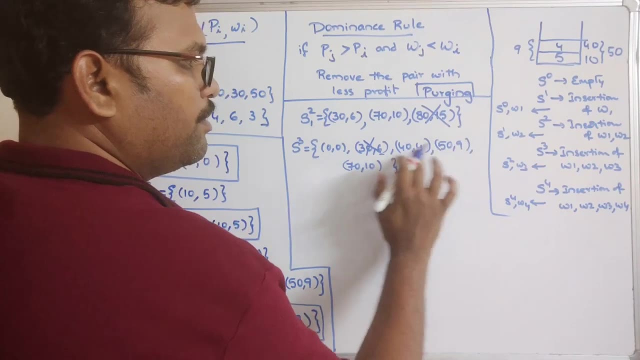 profit for weight 4.. So we can remove the less profit And see 0,, 4,, 4 to 9, and 9 to 10.. 0 to 40,, 40 to 50,, 50 to 70. Everything is the same, So we are getting a profit for. 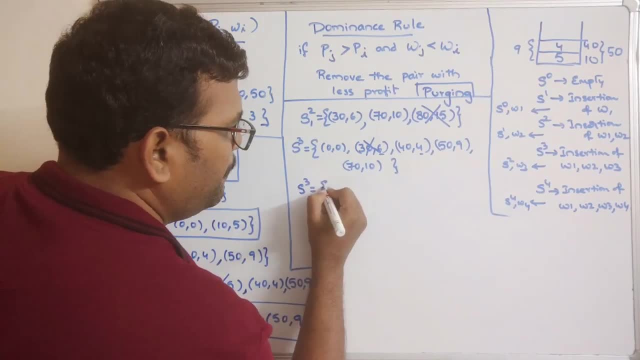 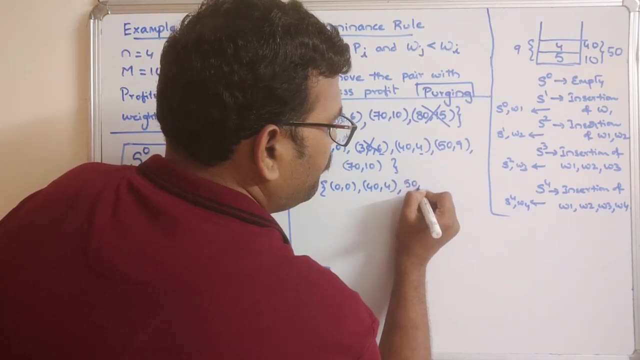 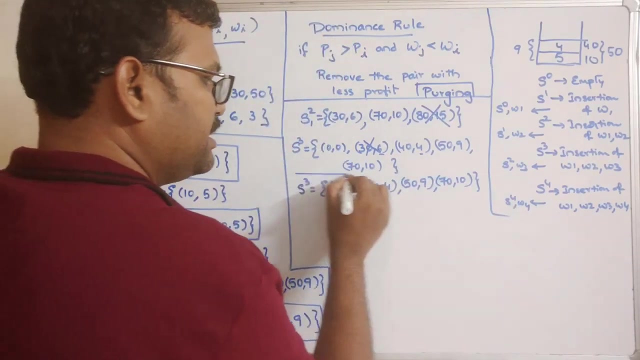 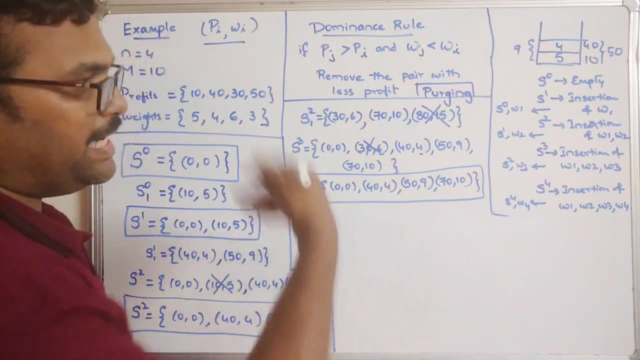 this. Okay, Now S3, the final S3, 0, 0,, 40,, 4,, 50,, 9,, 70, 10.. This is the S3.. This is the S3.. Now insert the last one. Already, we have inserted the three things We need. 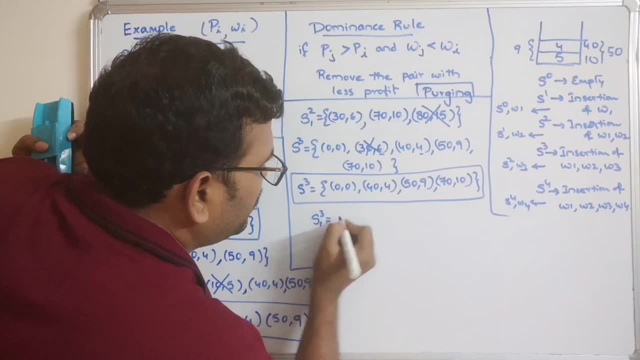 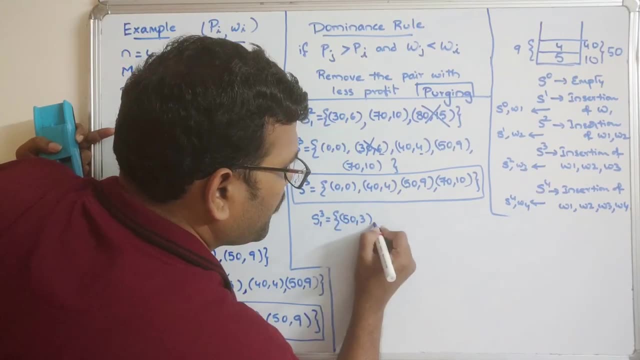 to go with the fourth one, So S1 into 3.. So we have to add the fourth one, So 50, 3.. So 50, 3, 53.. So 90, 7,. 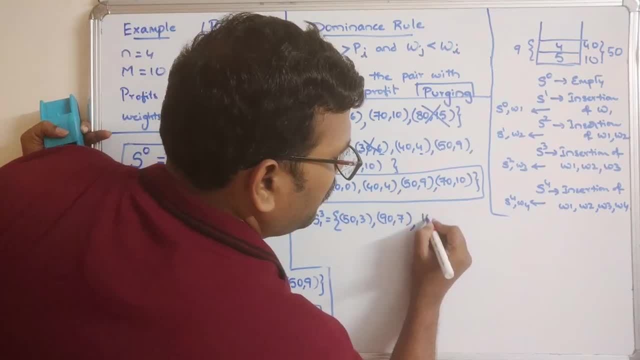 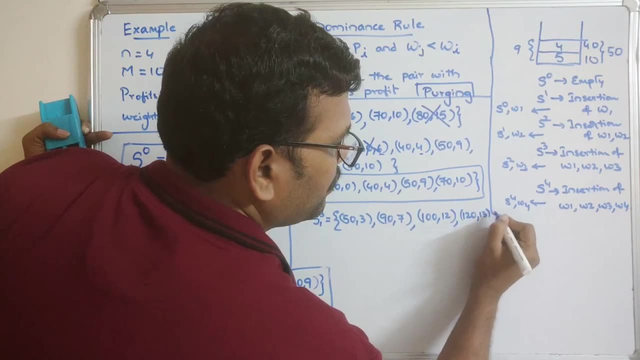 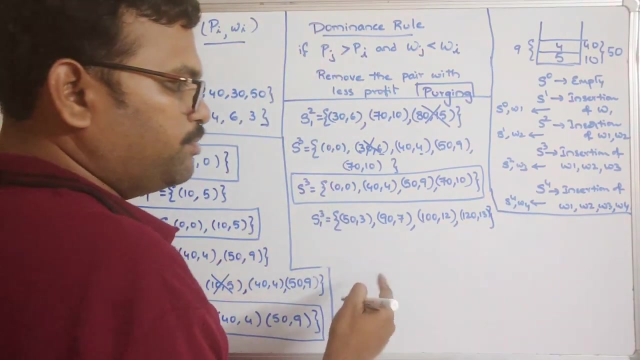 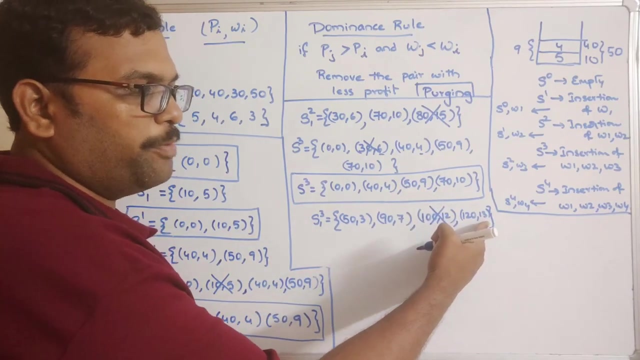 53, 53.. 100, 12,, 50.. 120,, 13.. Right, Okay, Now you can observe this is a beyond the weight 12.. So we can't process this one, And this is also beyond weight, Because 13 and the maximum capacity of those are only. 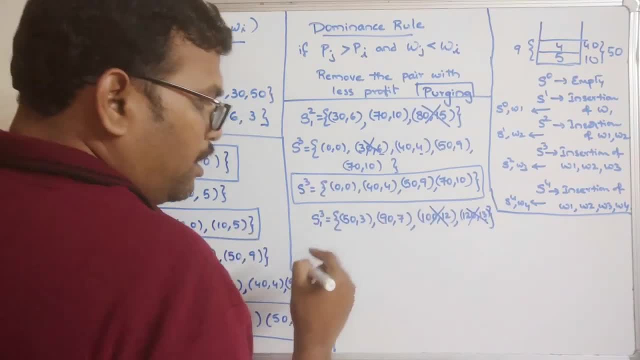 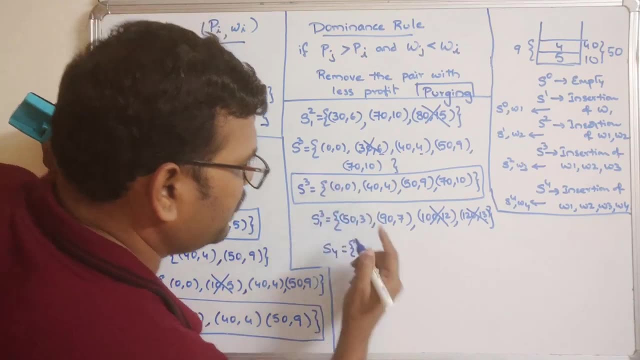 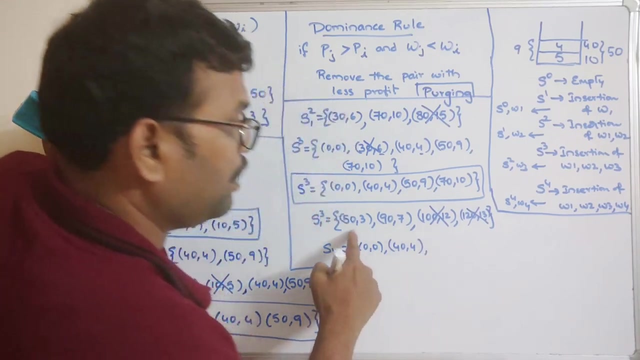 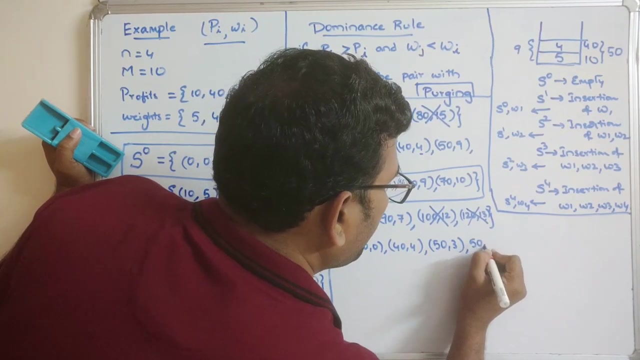 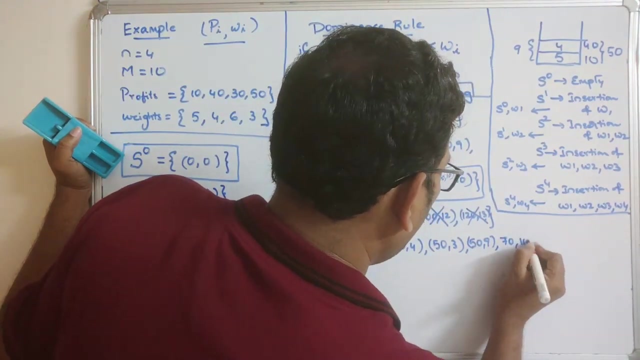 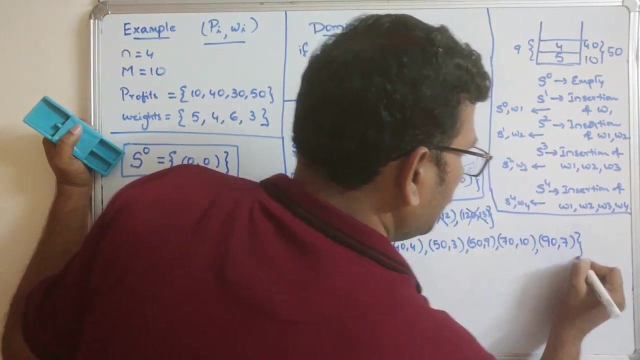 10.. So you can avoid this one. Okay, Now write on the S4. What is the S4?? Combine both the things, S3. So 0, 0,, 40,, 4. And you can go with the 50,, 3.. 50, 9.. 70,, 10.. 90,, 7.. See, these are the S4. And again, 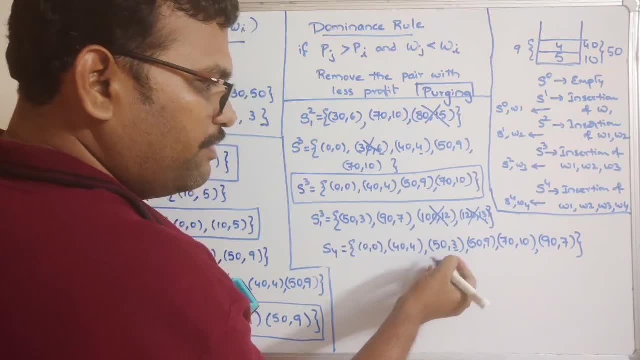 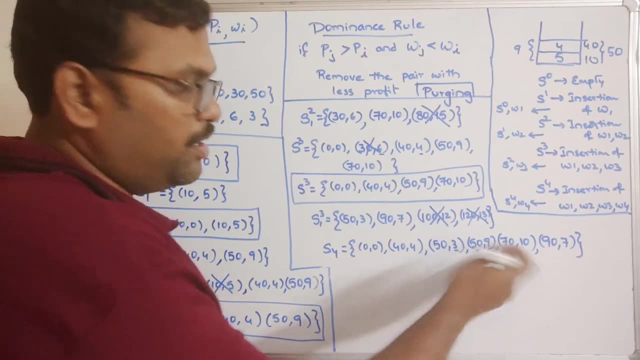 you can observe. Yes, So we are getting 3 with the 50 and 9 with the 50. Weight 3, 50, with the profit 50. Weight 9, with the profit 50. So you can avoid this one, Okay With. 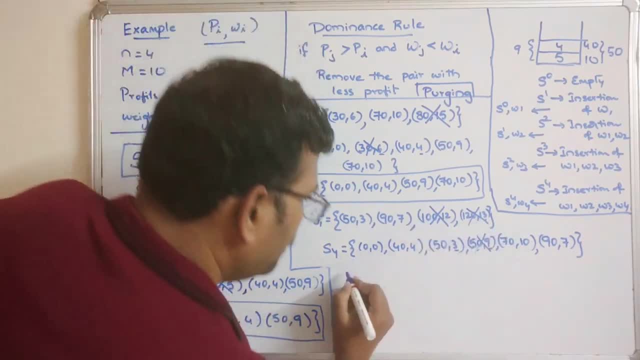 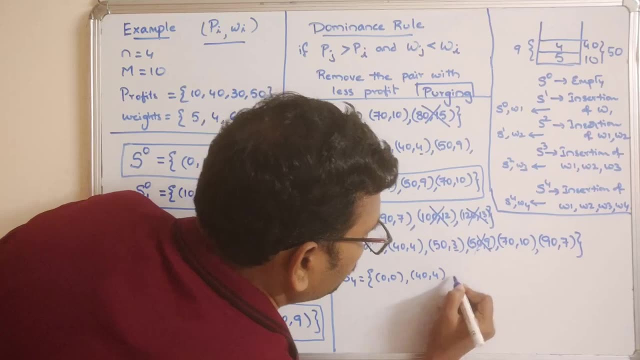 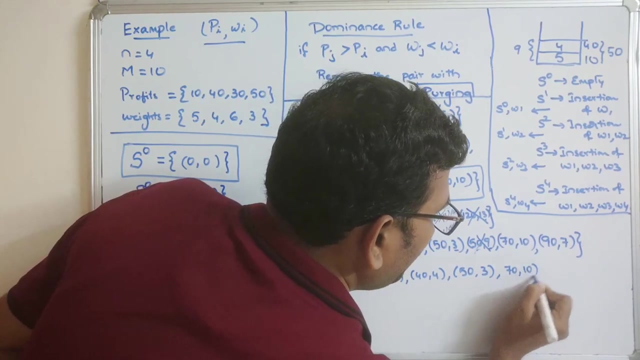 only weight 3, we can get a 50. Right, So we can avoid this one. So finally, write the S4.. 0, 0,, 44,, 50 and 3,, 70 and 10,, 90 and 7.. And again observe, So you can avoid. 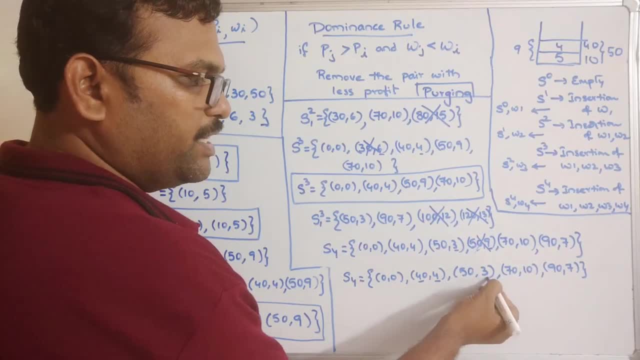 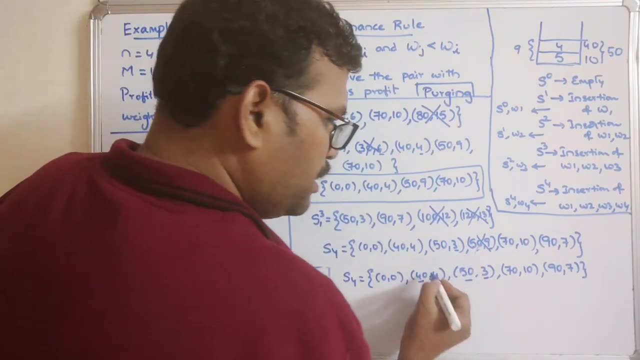 this one. So with 4, we are getting 40. And with 3, we are getting 50.. Okay, Again there is a violation. The same dominance rule, Right. So avoid the less profit, So you. 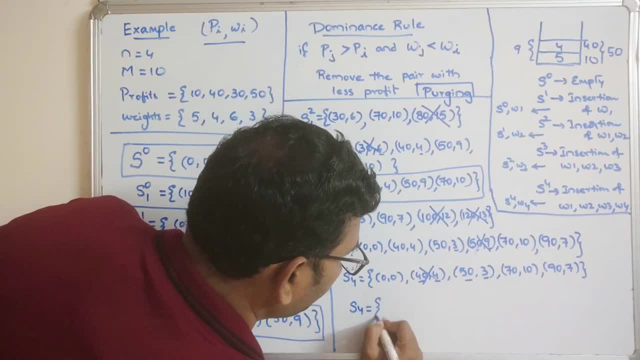 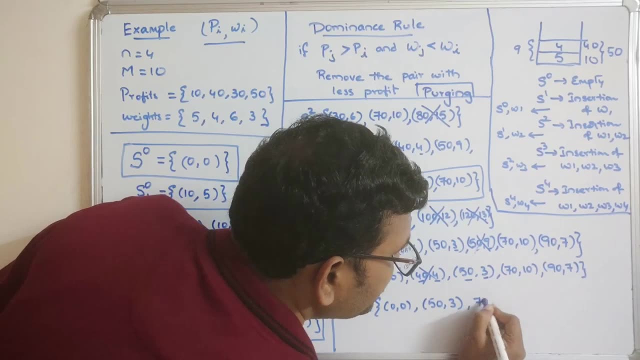 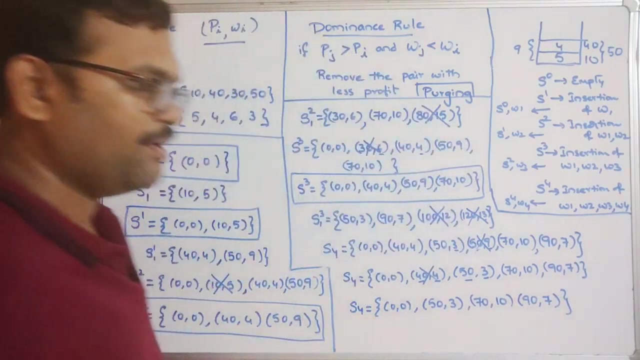 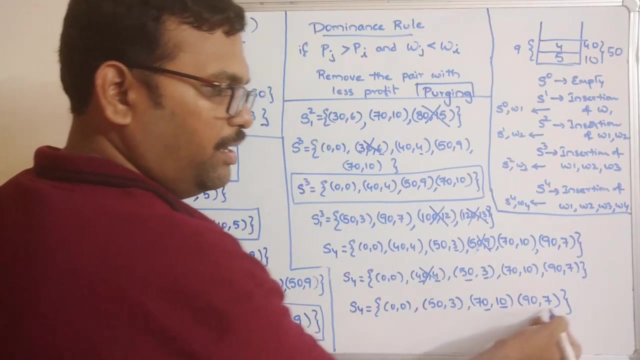 can avoid this one Again. write on the final thing, So hope you are understanding: 50, 3.. 70, 10.. 90,, 7.. And again you can see: So with 10 weight we are getting 70.. With 7 weight we are getting 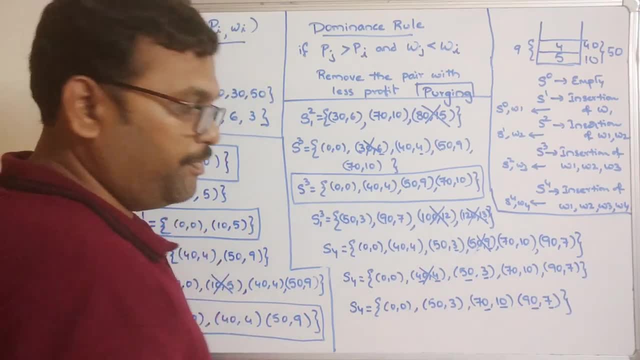 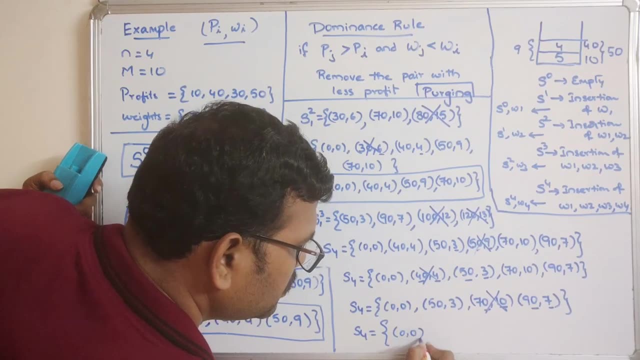 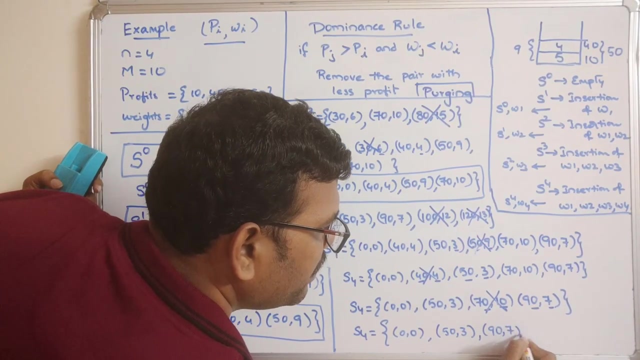 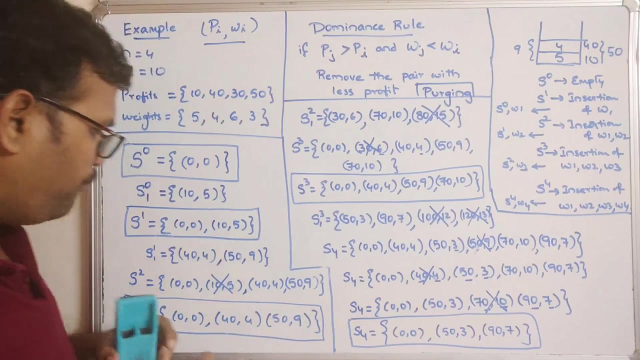 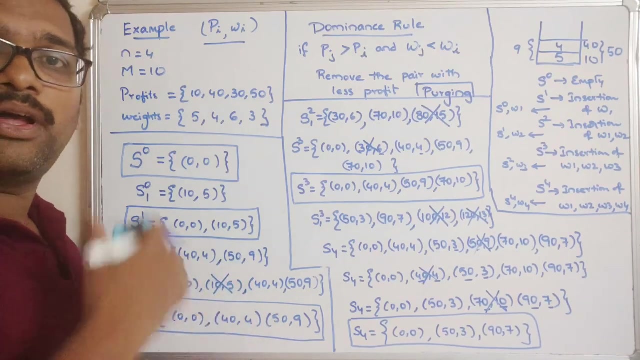 90. So again there is a problem, So you can avoid this one also. So S4, 0, 0,, 50,, 3, 97. So this is finally the S4.. s4- okay, so now we have found that s1, s2, s3 and s4, so we have inserted all the four elements. 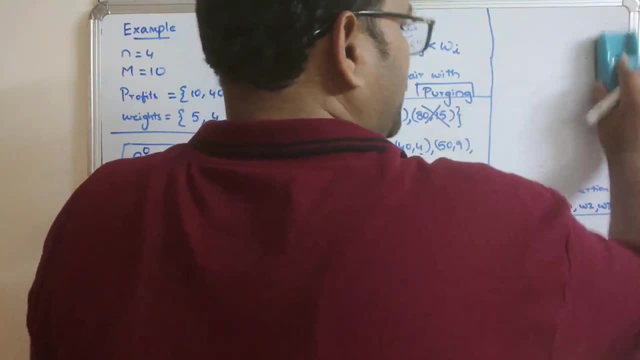 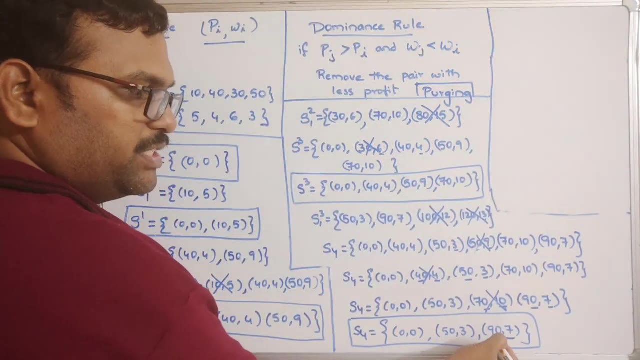 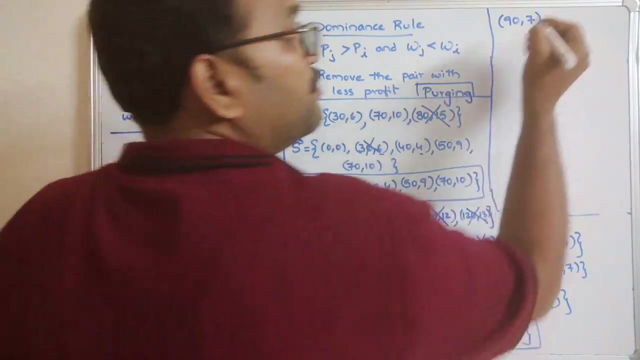 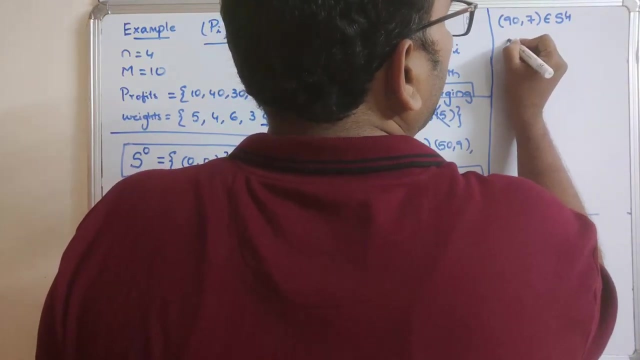 right now we'll see which one is the best, which one is the best among all these three. so here the highest is this one. so just consider the same thing. so 90 comma seven- check the conditions- belongs to s4, and 90 comma 7 belongs to. 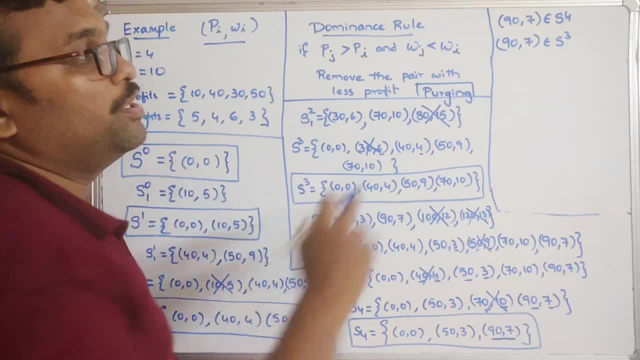 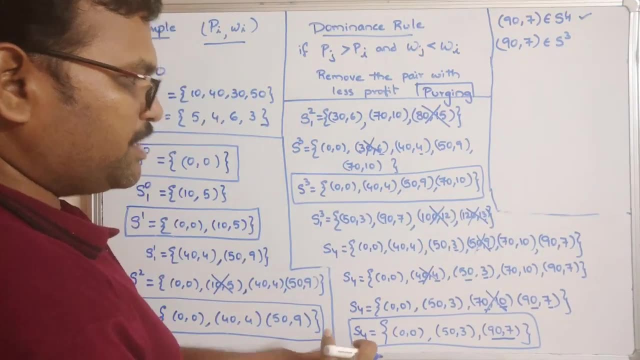 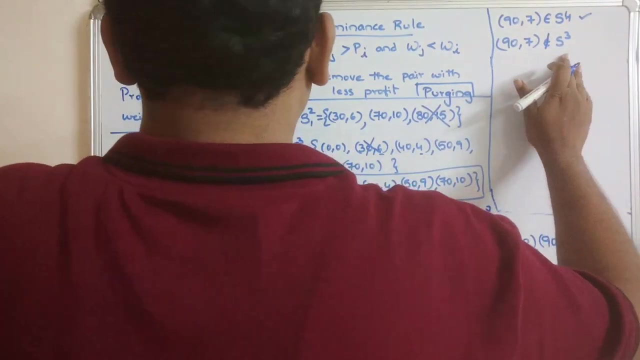 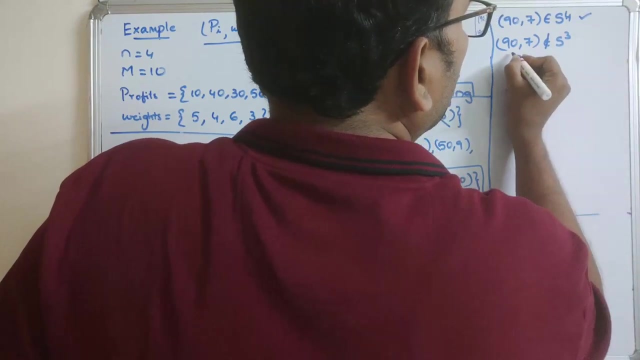 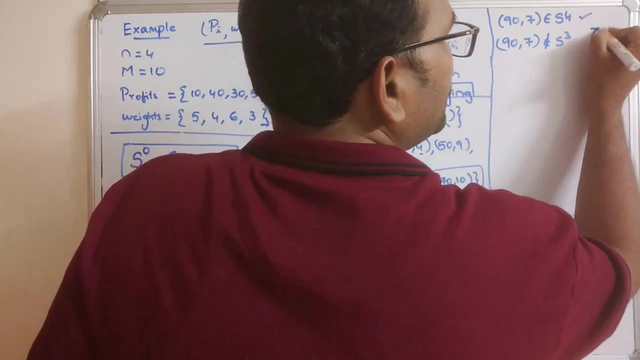 s3. check both the condition. okay. which one is true? so 90 comma 7: it is available in s4, right? 90 comma 7 is available in s3. it doesn't belongs in s3, okay? so here you can see: it is an s4, not in s3. that means you can simply say that. 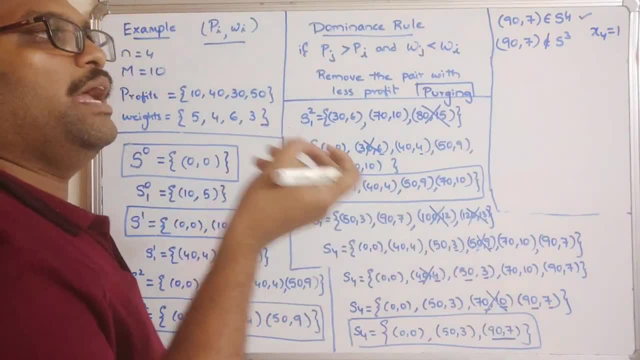 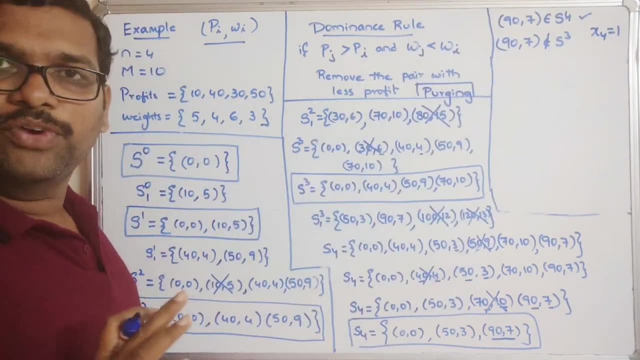 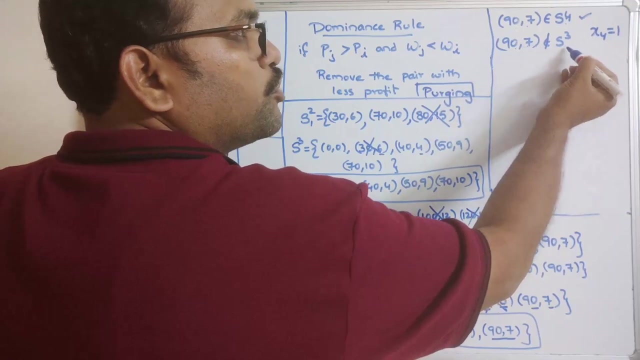 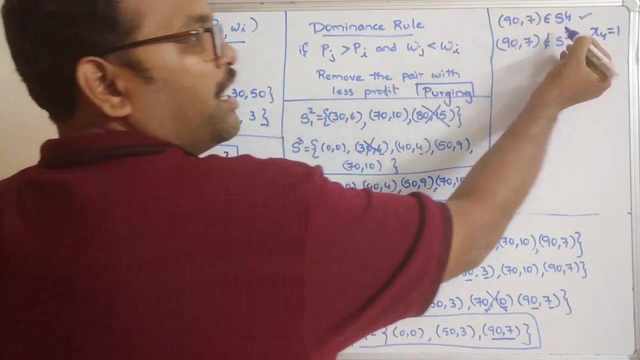 x4 is equal to 1, that means we can move the element into back into the sack. okay, if both are equal, we need not move it. okay, both are equal. that means if 90 comma 7 is it belongs to s4 and 90 belongs to s3, then we need not move the weight to the sack. so here one condition is true, another. 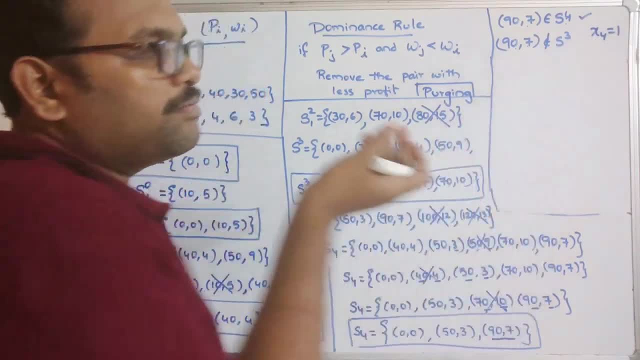 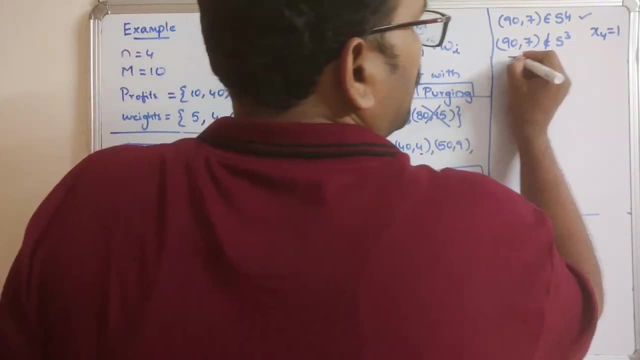 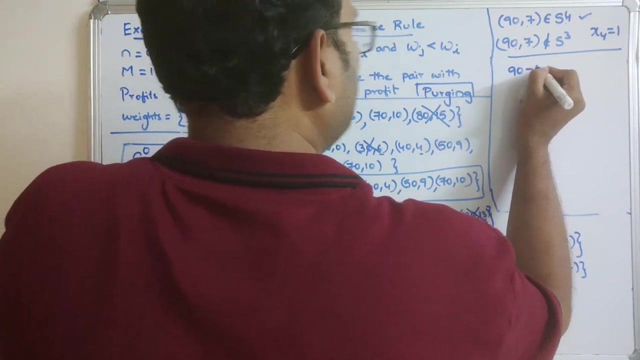 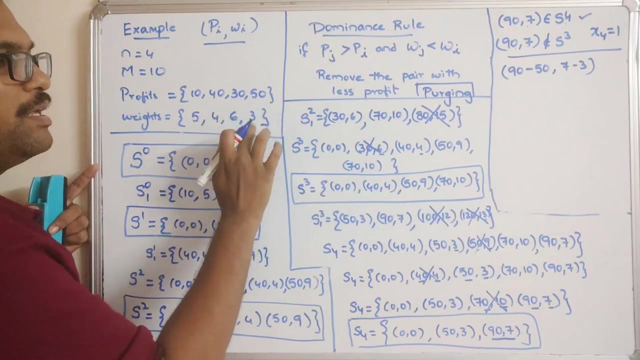 condition is false. so move the fourth element, last element or last weight into the sack. now remove the fourth element from this particular weight. so 90 minus 50 comma 7 minus 3. so this is the fourth one, 50 comma 3. so remove the things from the peg. so obviously. 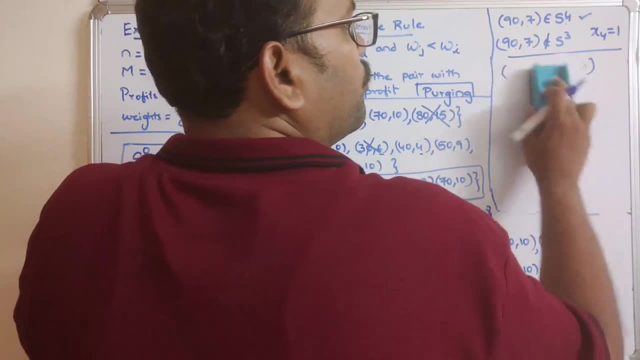 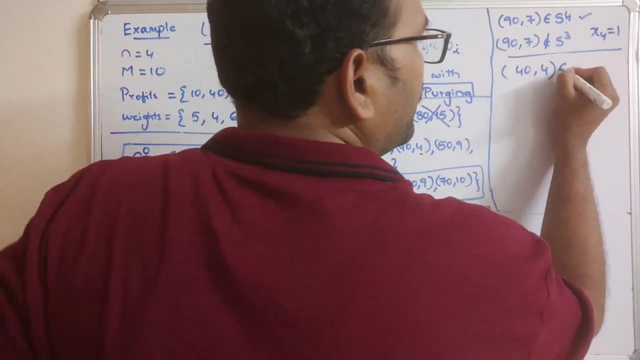 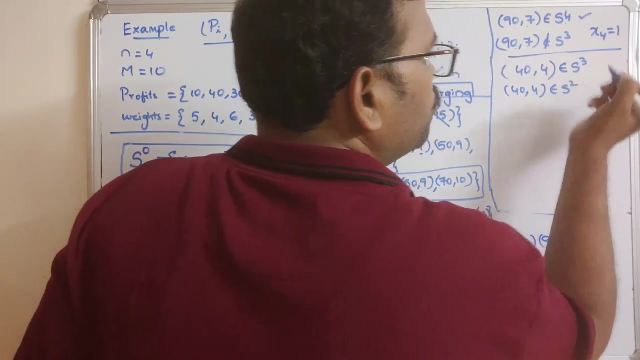 it will be 40 and 4. check out so 40 and 4 check the same conditions. now already s4, completed, belongs to s3 and 40 comma 4 belongs to s2. check out whether 40 comma 4 belongs to s3. 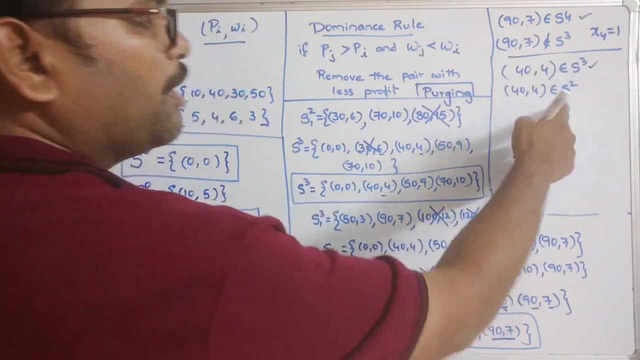 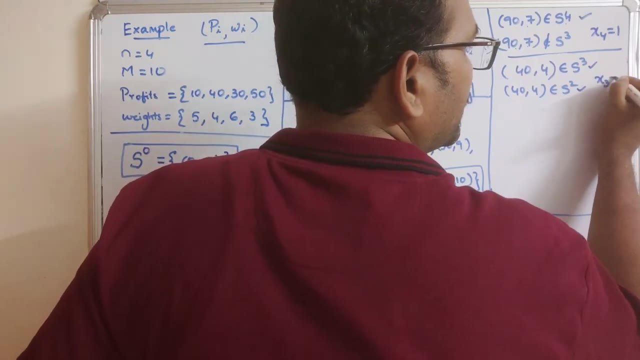 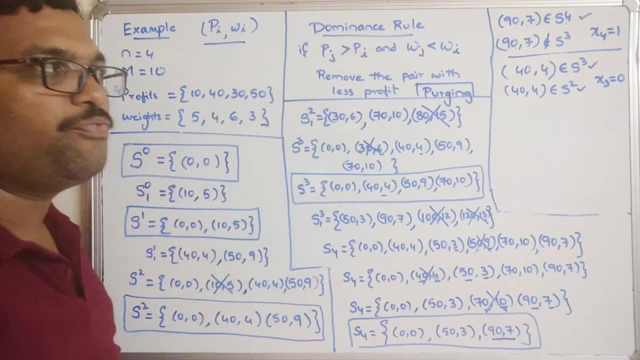 40 comma 4. it is available, right, 40 comma 4 in s2. where is s2? 40 comma 4 in s2? yes, so obviously we can say the third object need not be moved because both the conditions are true. so in both the cases, in the both the sets, 40 comma 4 is available. so need not change. so in our first 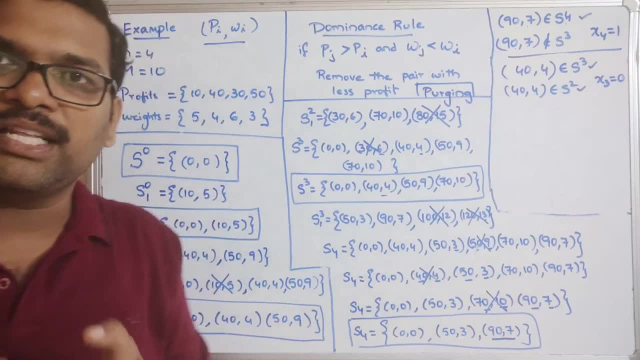 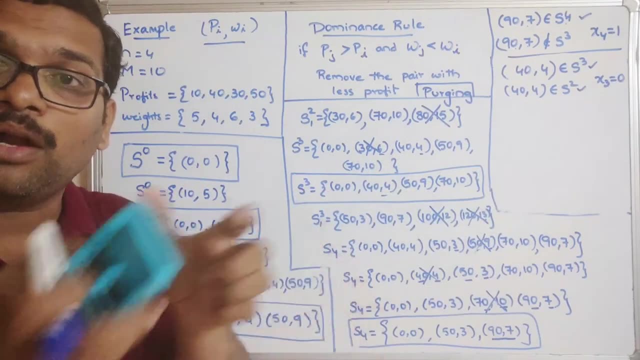 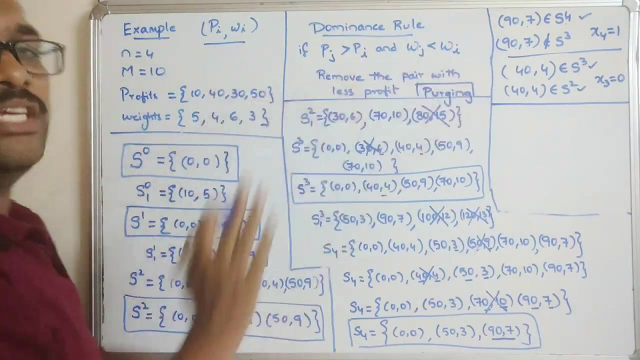 discussions, we say that one represents moving the sack into the. i mean moving the weight into the- and coming to the zero representation. we should not move the weight into the set then. so we did not remove the third element from this here. okay, so simply continue with the same thing. 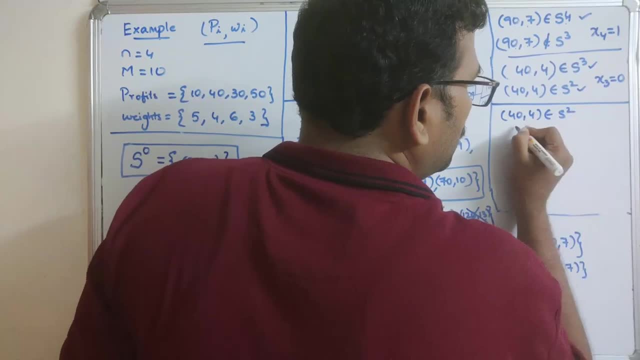 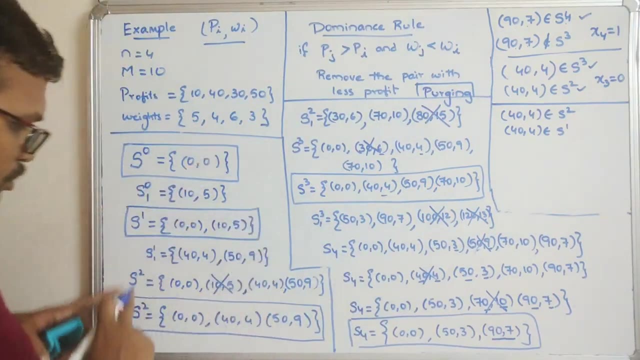 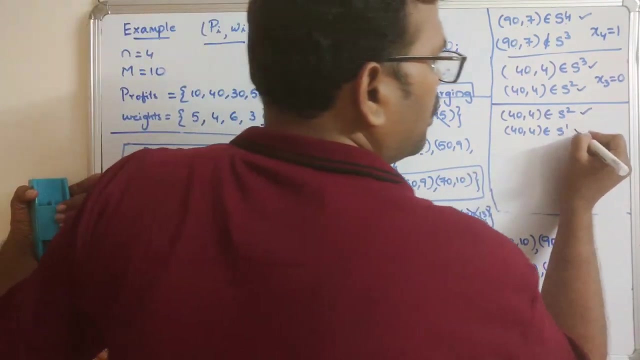 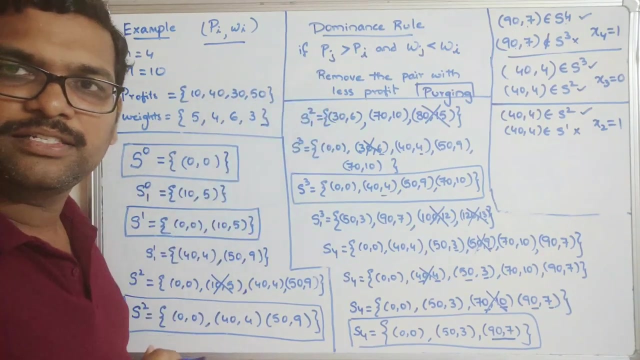 so 4 comma 4 belongs to yes 2. 40 comma 4 belongs to s1. check out in s2 40 comma 4, it is available. 40 comma four in s1: no, not available. so that implies x2 should be moved. x2 should be moved into the set. hope you understood if both. 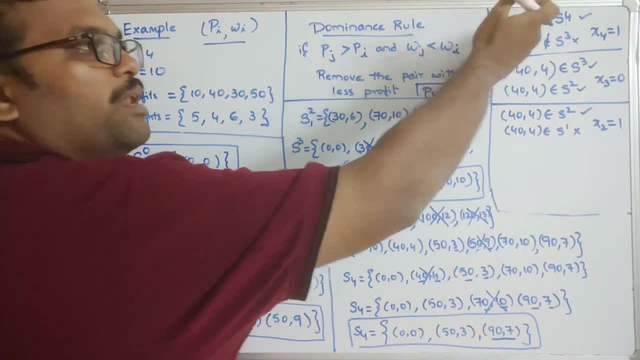 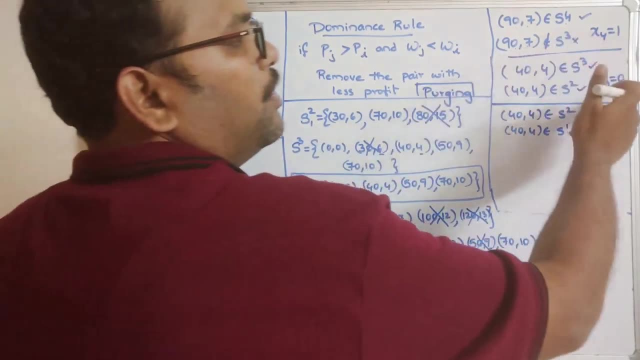 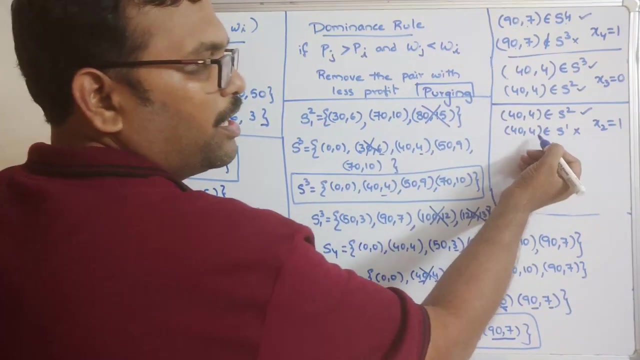 the conditions are true. that means if the pair is available in s of i and s of i plus 1, or sorry, s of i minus 1, then then no need to move the weight into the set. so we need to compare each and every set. okay, so here, 40 comma 4 is available in s2 and 40 comma 4 is not available in s1. 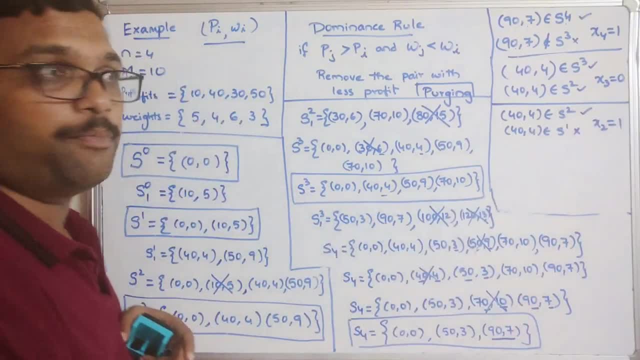 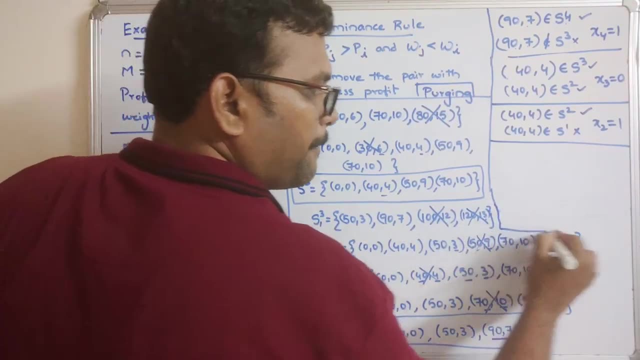 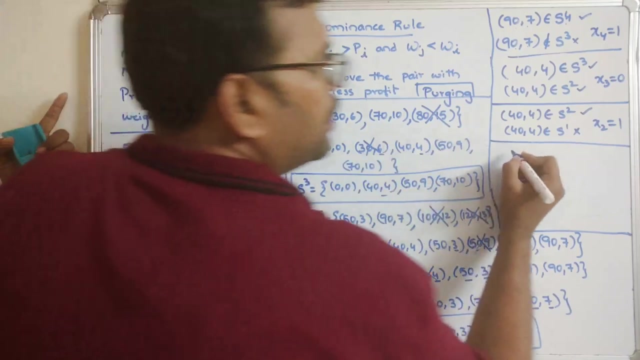 so that's why we have to move the second weight, because we are checking with the second one right now what happens. so here we need to remove the second element from this pair. so what is the second element? 40 comma 4. so 40 comma 40 and comma 4 comma 4. 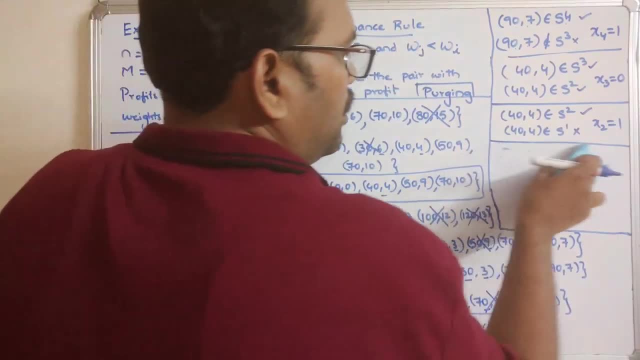 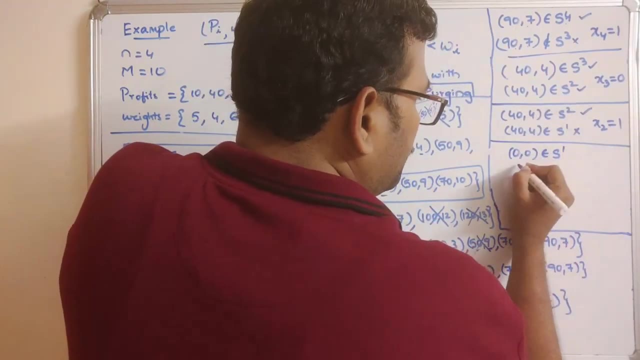 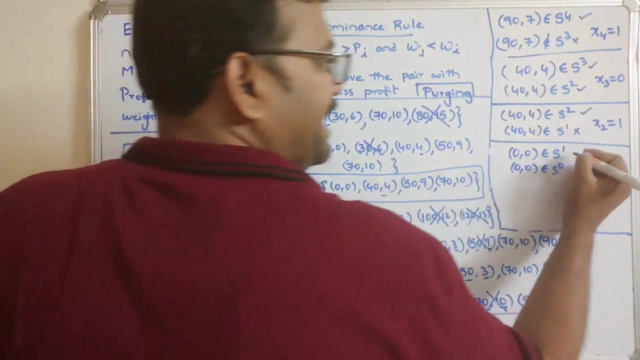 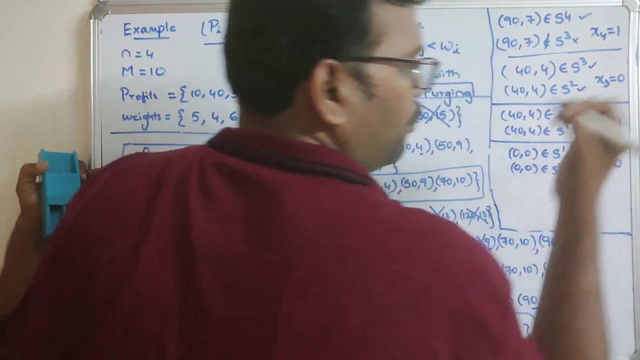 So what happens? 0, 0.. So it is 0, 0.. So we have to check again with 1 and 0, 0, with S naught. So 1, 0, 0, yes and S naught 0, 0, yes. So obviously X1 will be 0 because the pair is. 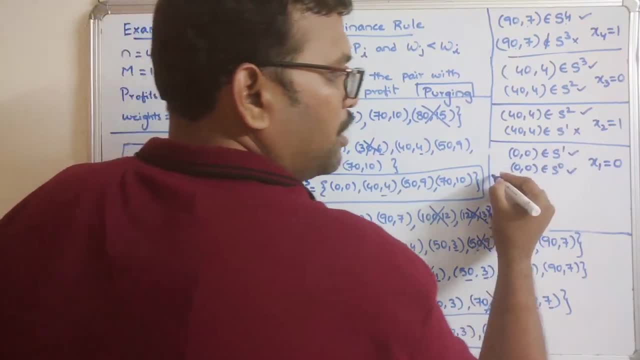 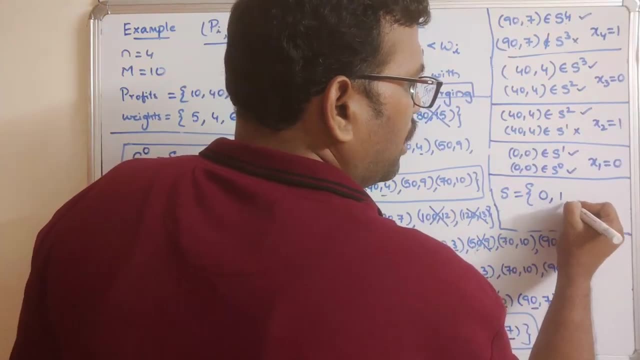 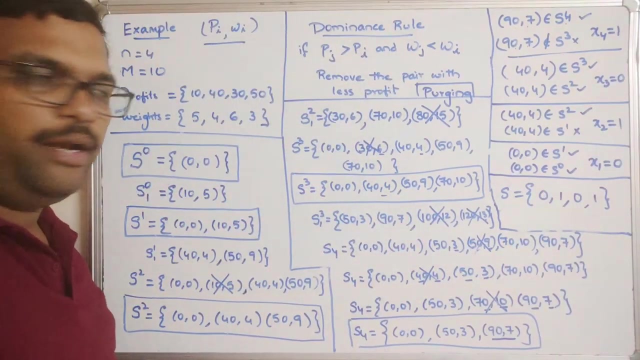 available in both the set S1 and S naught. So the solution is 0, 1,, 0, 1.. So the solution will be either 0 or 1.. So 0 means we should not move the first weight, 1 means we have. 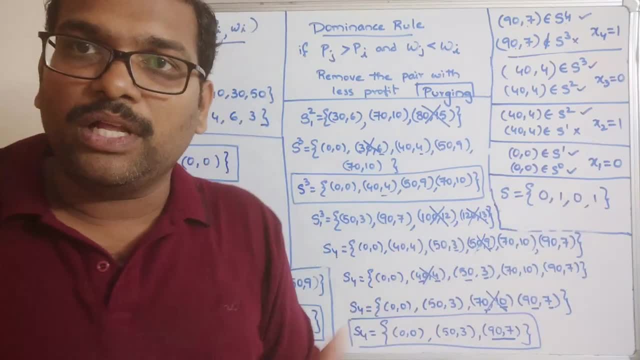 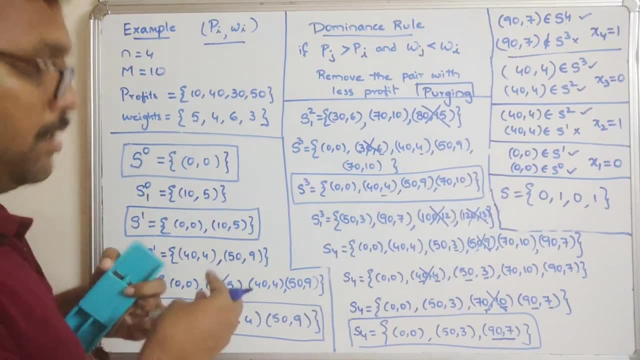 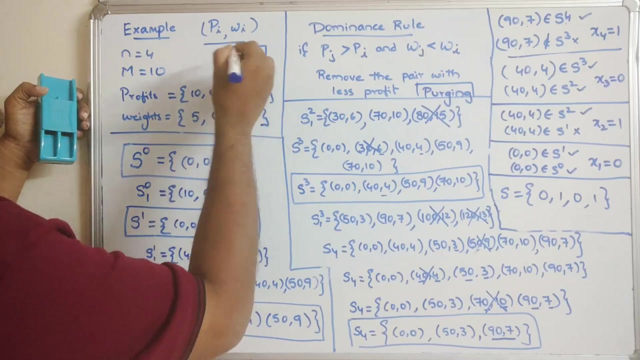 to move the second weight. 0 means we should not move the third weight And 1 means again we have to move the fourth weight. Just observe, moving of. see, this is a weight, this is a weight Moving of second, one second. 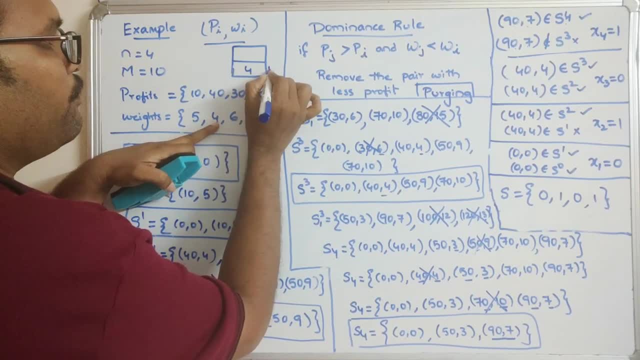 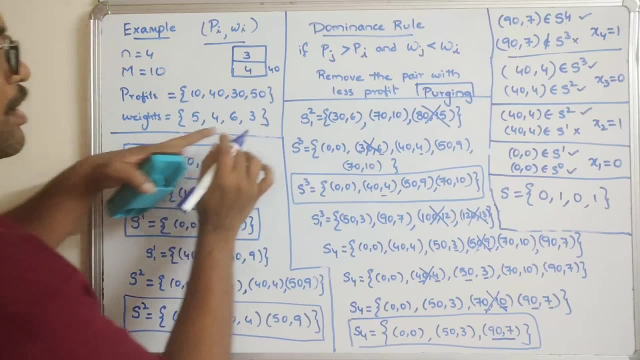 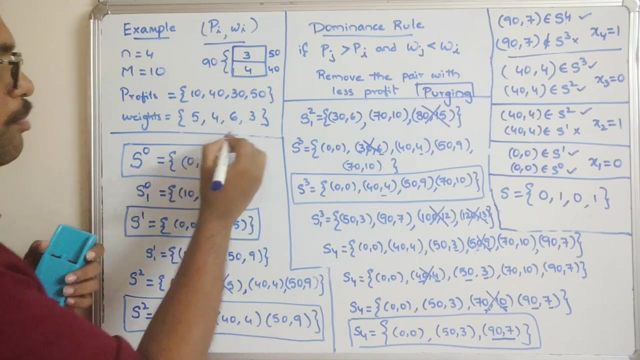 weight is 4, with a profit of 40.. Next, third, fourth. fourth means this: one Third weight, okay, with a profit of 50.. How much total profit? we got 90.. 90 profit. So, moving by moving a 3 and 4, okay, by moving a weights 3 and 4, we got. 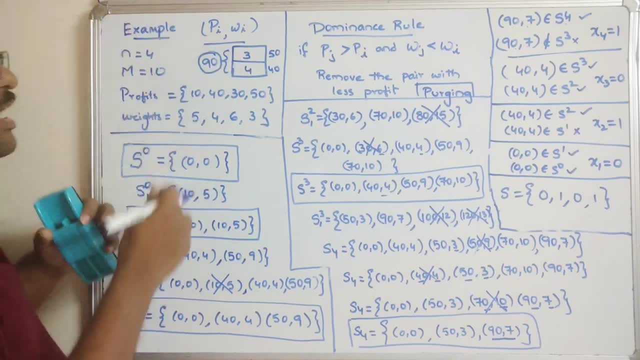 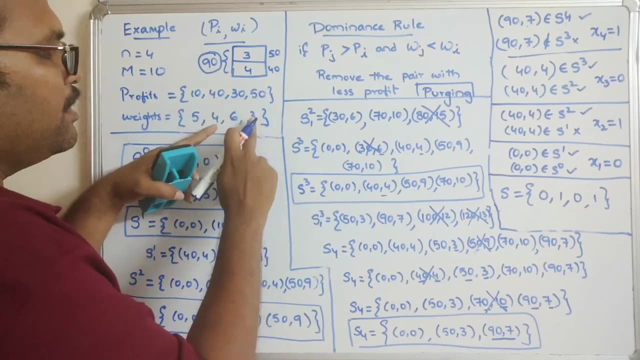 a 90 profit. That is a maximum profit. You can check. So 5, 4,, it is 50.. 4, 6, it is 70.. 6, 3, it is 80.. 3, 4, it is 90.. Just now we got it 5, 3, 60.. In every combination. 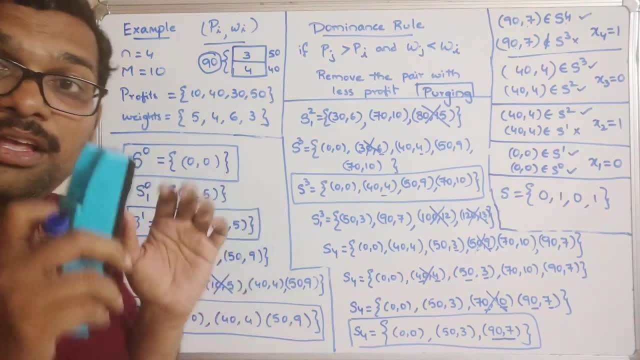 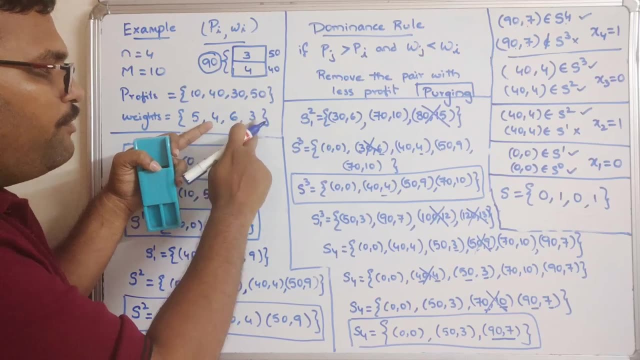 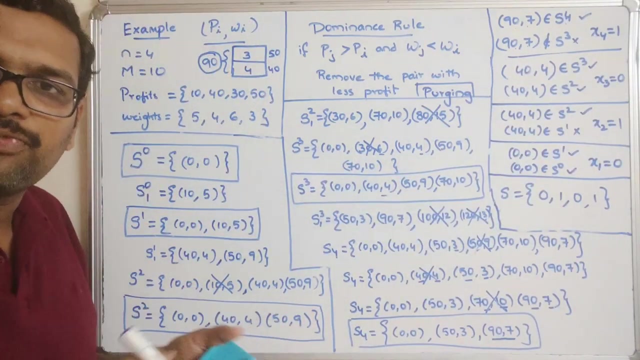 you can check. So only, we will get a maximum profit If you move the third weight and the fourth weight, sorry, the weight 4 and weight 3, that means the second and fourth one, So x2 and x4.. If you move the x2 and x4 weights into the 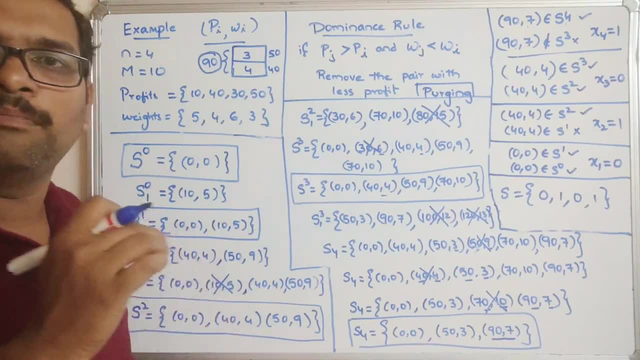 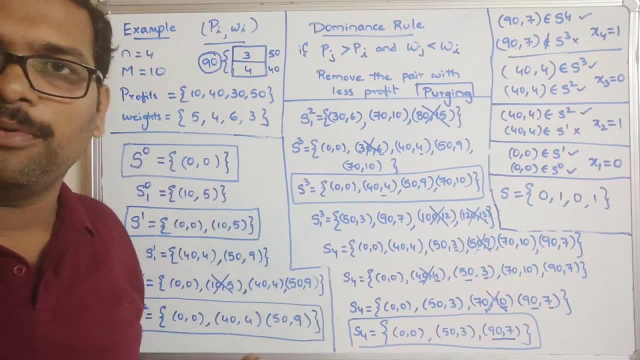 sack, then only we will get the maximum profit. Okay, So this is how we can solve the knapsack problem. So first we have discussed about what is a knapsack right, And then we have discussed how to solve the knapsack problem. So first we have discussed about what is 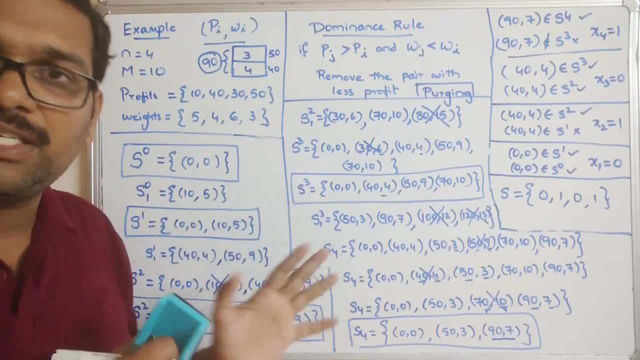 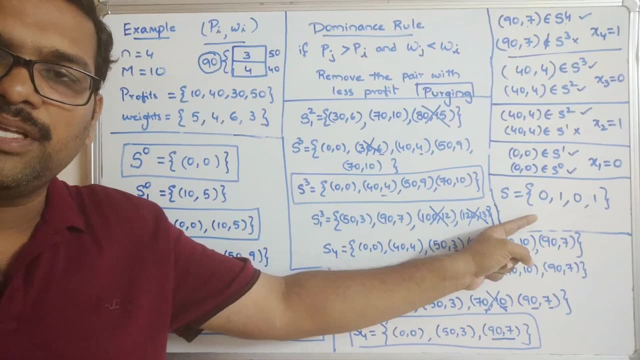 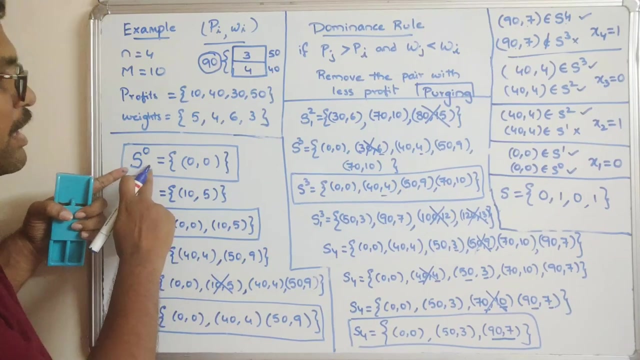 a knapsack problem, right? This is by using the set method. By using the set, we are using all the combinations and then, simply, we are getting the result with the zeros or ones which are to be moved and which are not to be moved. So, once again, I am repeating: So. 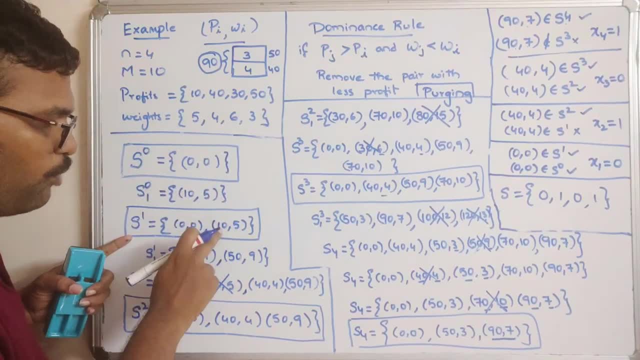 initially insert one element and then insert the initially the sack will be zero. and insert one element and combine both the things and insert the second element and combine both the things and just put together like this: First you can engine own the change value of the same to a null. So again, once you yourself do that, you know the industry is in a mental 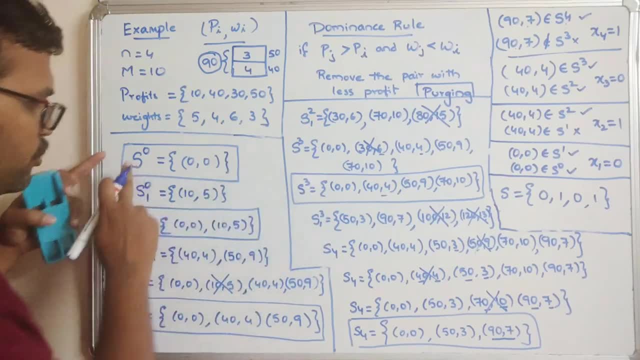 crash. So you just need to see how it works and you just need some questions, right, And then you can again for free. Okay, Now, basically you can filter out soil in the first half медium, just remember. so make it a mark of S0, S1, S2, S3 and S4. and one thing we have to remember: 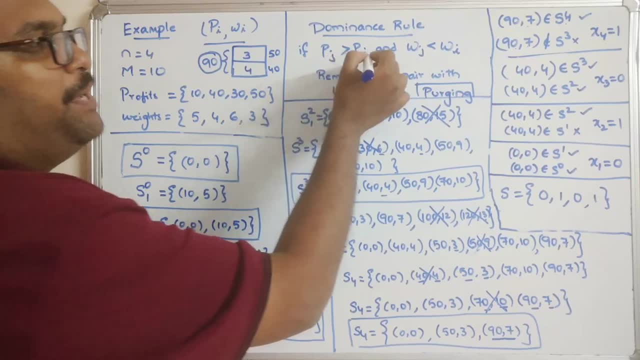 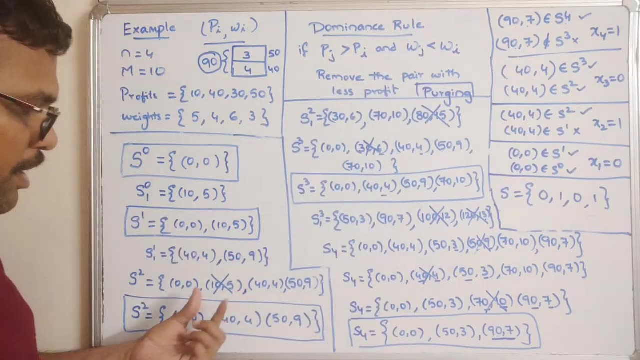 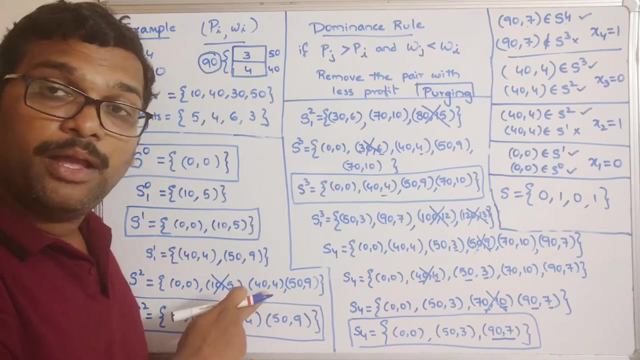 the dominance rule. if the PJ greater than PI and WJ less than WI, then immediately remove the pain with the less profit. Simple example: we are inserting weight 5 and we are getting a profit of 10. and we are inserting weight 4 and we are getting a profit of 40.. So here, 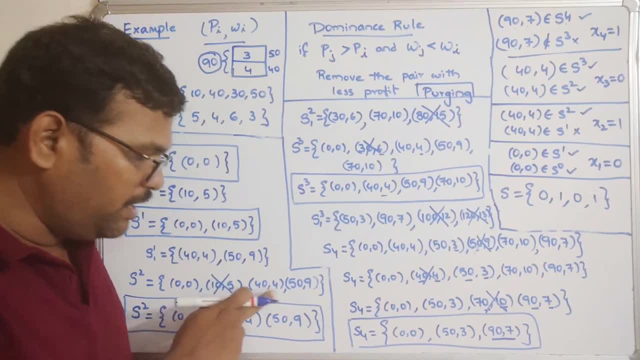 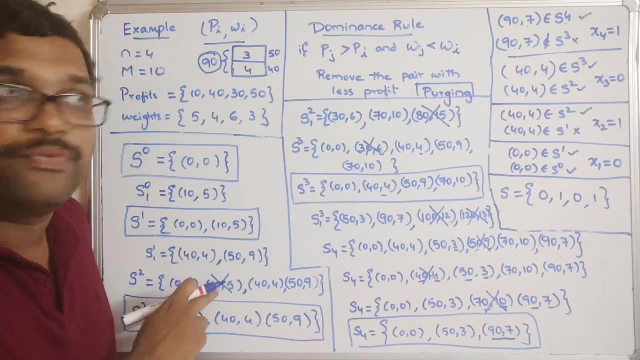 the remaining weight we can insert into a bag is only 5, and in this case we can insert the weight of 6 into the bag, right? So that means with the highest weight we are getting a lowest profit. So such cases we can remove the pain with low profit and that we call. 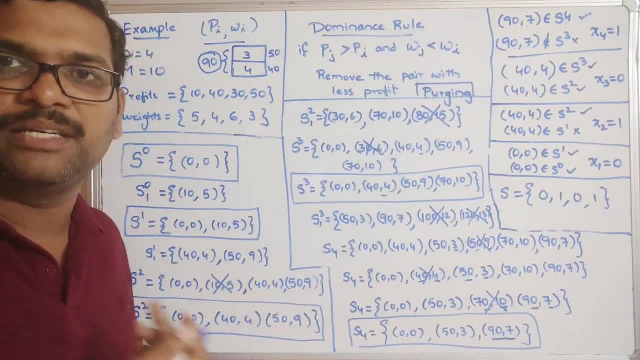 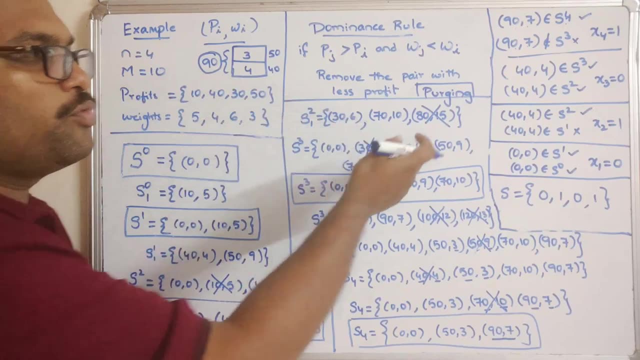 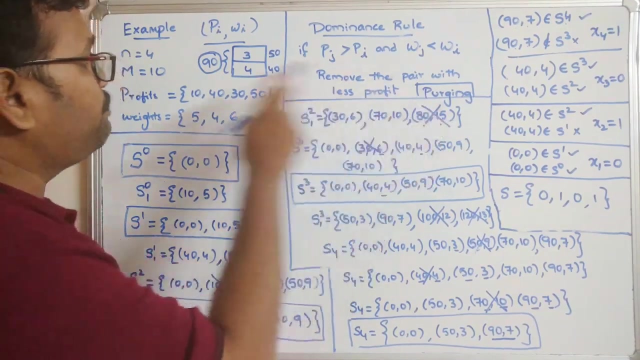 it as a dominance rule or the technique called a purging mechanism. And one more thing: so if the weight exceeds the maximum size, then also we can remove the weight. So in this case we can remove the pain. Here you can see 80,, 15.. So 15 is the weight which is beyond. 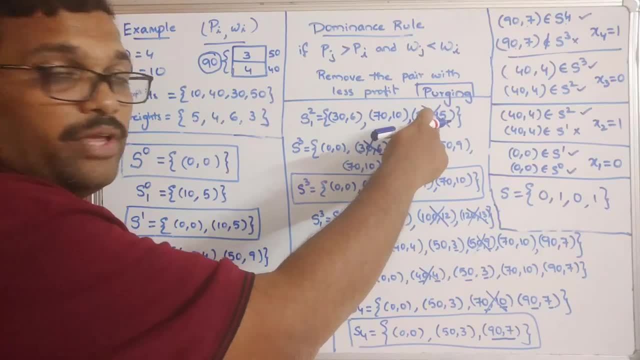 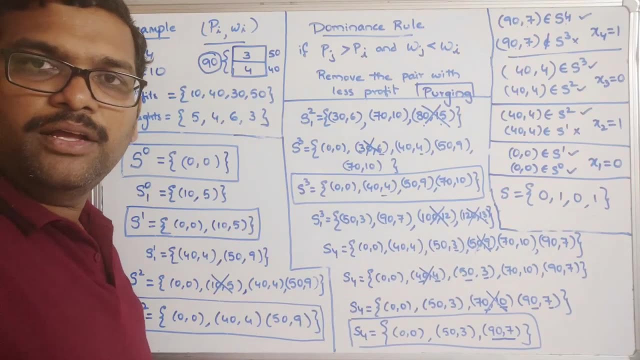 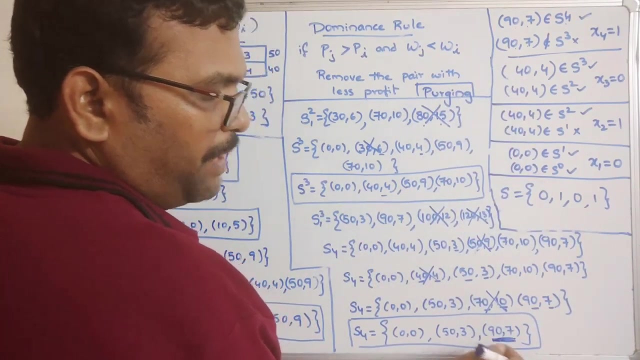 the maximum. So we have avoided it, We have ignored. So here, in this case, 12 and 13, we have ignored right and all these are the purging. Okay, so dominance rule: applying the dominance rule Afterwards we need to check the highest weight or highest profit. pain with the S4. 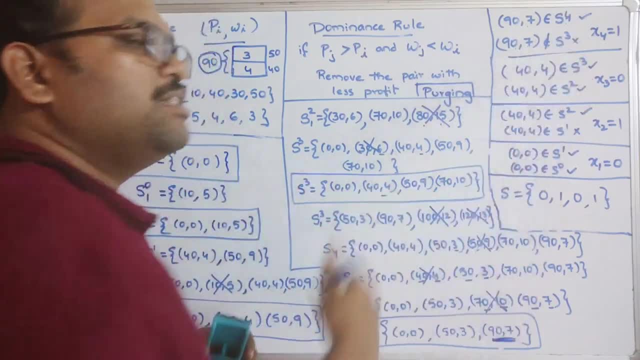 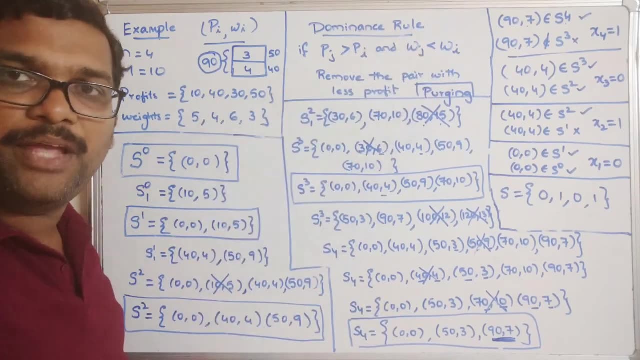 and S3. So that if it is belongs to in both the case simply we can say we should not move it because already in either cases- I mean in some other case it may be available- So automatically we should not accept it if the pain is available. 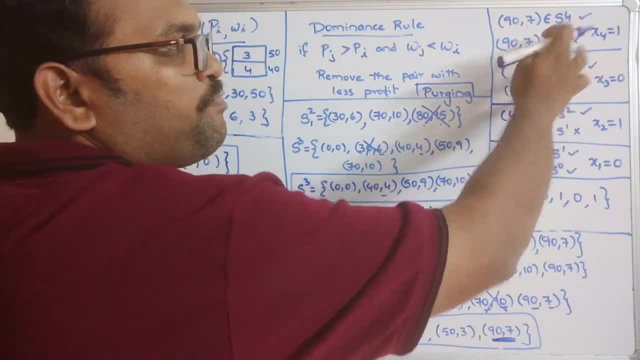 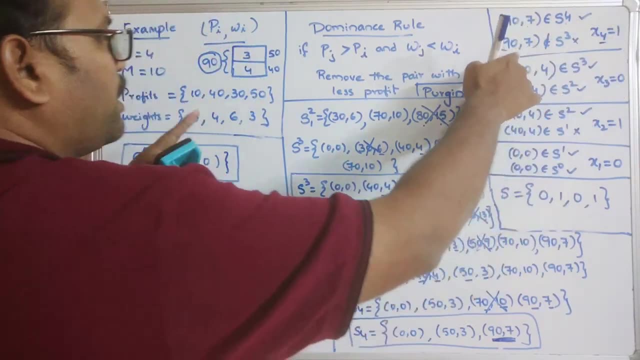 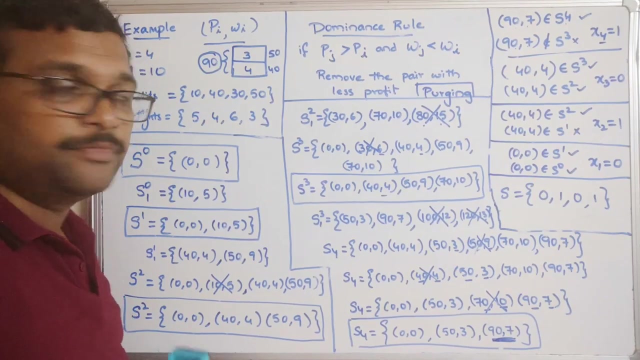 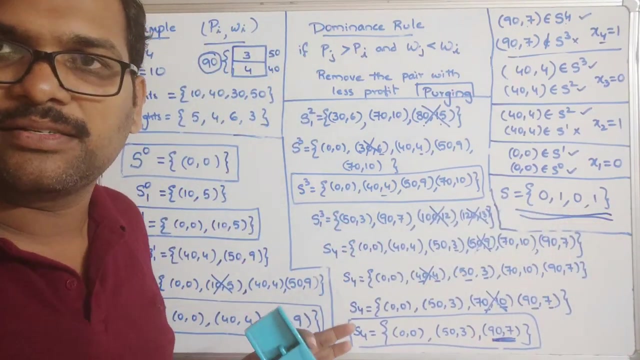 in SI and SI-1.. And if not, then immediately we can move that particular weight and we have to remove the fourth, that particular weight and profit from this particular weight. profit and weight pain, Right, so like that. finally, we will get the solution in either only 0s or 1s. So this represents: 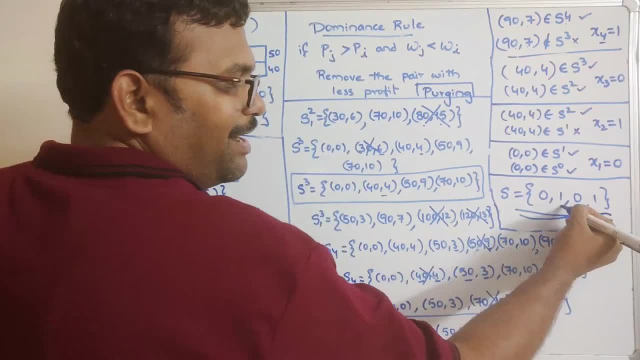 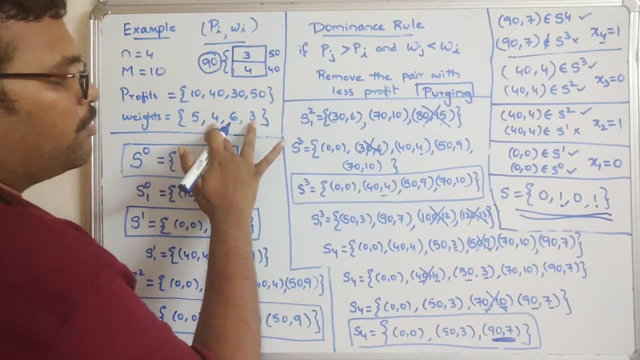 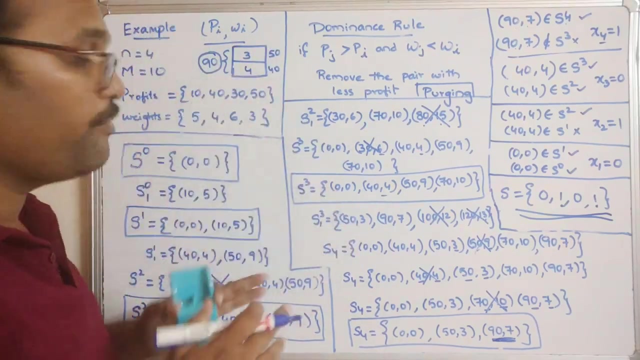 we are moving. so by moving the second object and a fourth object we will get the highest profit. By moving the second object 4 and third of sorry fourth object 3, we are getting the maximum profit of 90 rupees, So 90.. Profit as 90.. 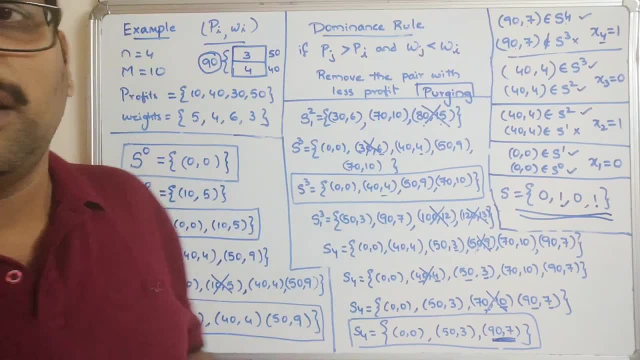 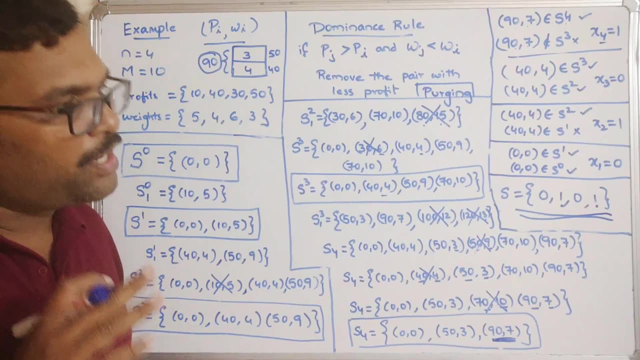 Okay, so this is how we can solve the 01 knapsack problem, Right? so hope you enjoyed and hope you understood the thing. So just practice a few more so that you will be confident about solving this 01 knapsack problem, Right? so let us stop here. If you are having any doubts, 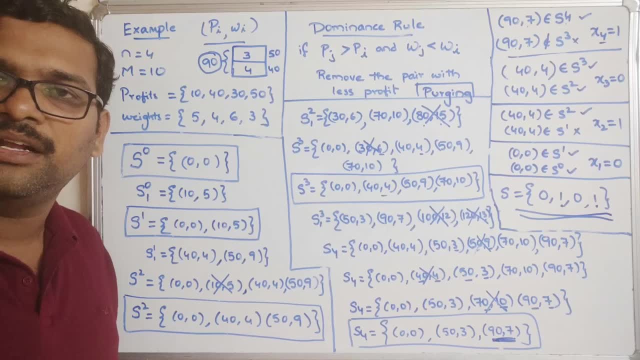 regarding this procedure, so feel free to post your doubts in the comment section. Definitely, I will try to clarify all your doubts. If you really enjoy this video, please do like it and share it with your friends and family, And if you have any doubts regarding this, video. please do not hesitate to post your doubts in the comment section. If you really enjoyed my session, like my session, share my session with your friends and do not forget to subscribe to our channel. Thanks for watching. Thank you very much.